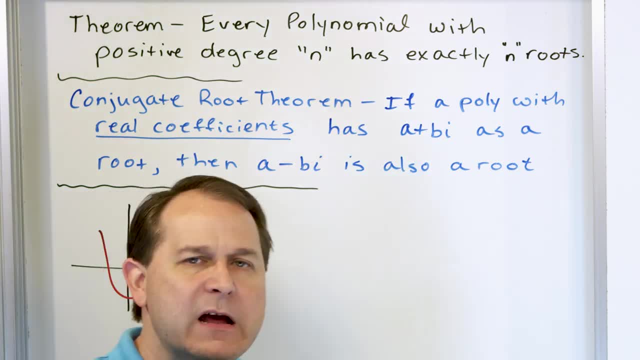 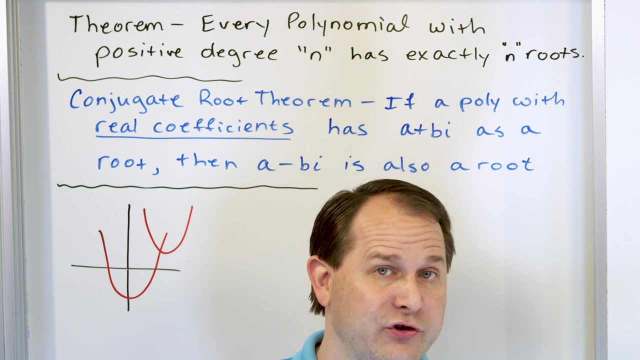 you'll see that the polynomial might exist up here, where there's no crossings on the x-axis, but that's okay. That just means that there'll be two complex roots. But no matter how you slice it, every quadratic is going to have a degree of 2. And because of that it will have two roots. 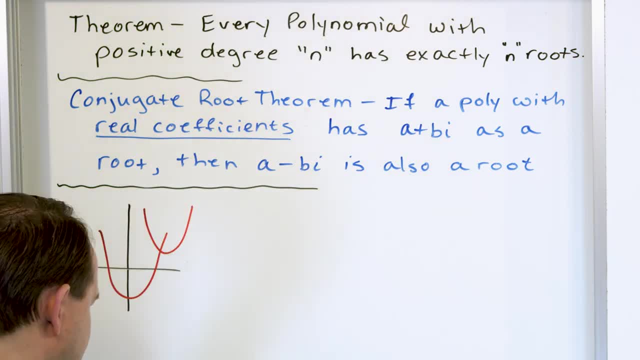 either two real or two complex roots. Going up one more, you can see that we have the cubics. We've talked about this in the past. A cubic is a degree of 3. It means x, cubed, plus some other terms. In general, a cubicle looks something like this, So you can see 1,, 2,, 3,. 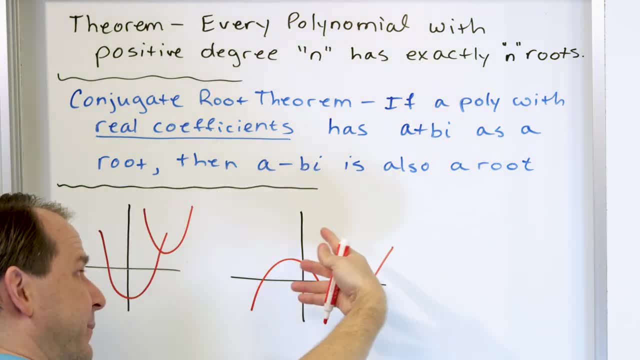 4, and 5.. So if you have a cubicle, you have a degree of 3.. But if you have a cube, you have a degree of 3.. So you can see that you have two crossing points, And of course it might be. 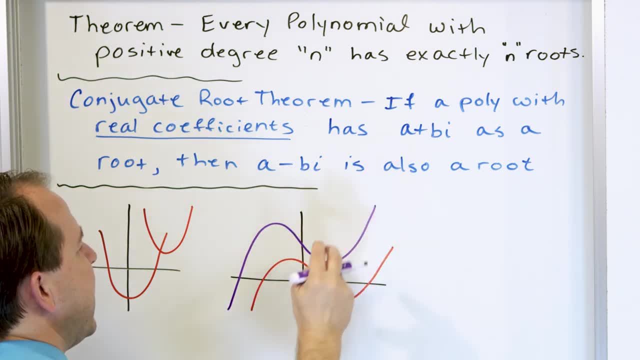 flipped upside down so it goes up and down the other way, but it will cross in three locations. If you have a weirder cubic that maybe don't have three crossing points like this, it might cross like this and then go down and maybe it doesn't cross on the second and third time. In that case, 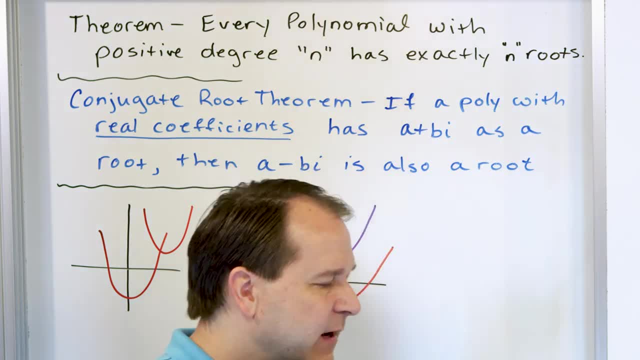 you would have one real root from this crossing And this one since it doesn't cut through the actual axis. those would be two complex roots, But you would still have a total of three roots, some real, some complex. We'll do one more. 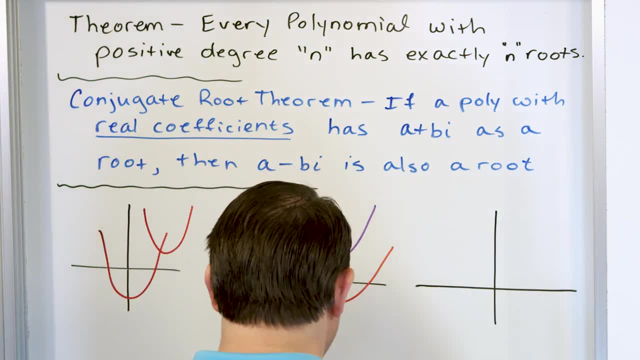 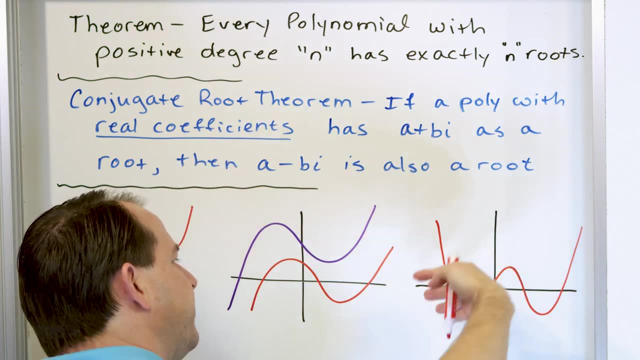 just to make sure you understand, because it's been a while since we've talked about this stuff. But a fourth degree polynomial in general will look something like this: So it'll go down, up, down, up. Of course, it could be flipped upside down and so on And you can see that there's four. 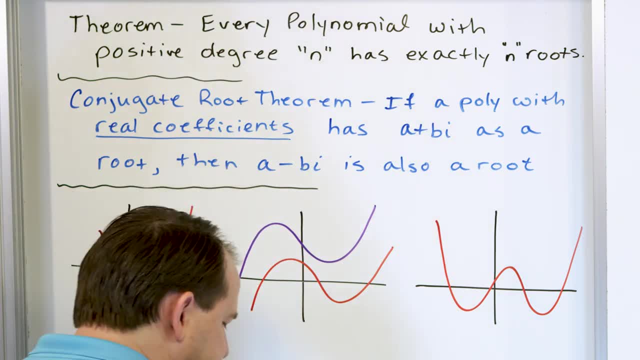 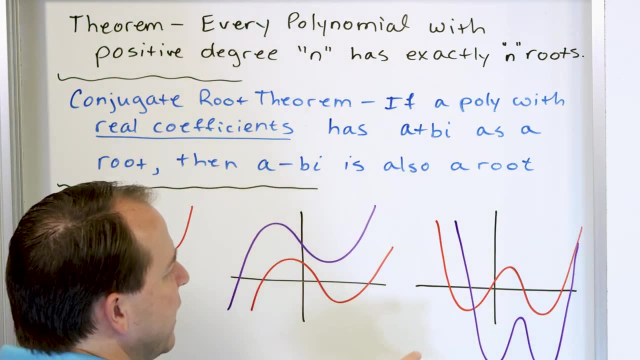 crossing points there. Now, of course, you can have other variations on that, where, for instance- let me do this one in purple- You might go down and then up and then down and then up again, something like this. So you would have one, two real crossing points. These guys didn't really make it up to cut through. So those other four roots would go up and then down and then up again, something like this. So you would have one, two real crossing points. These guys didn't really make it up to cut through, so those 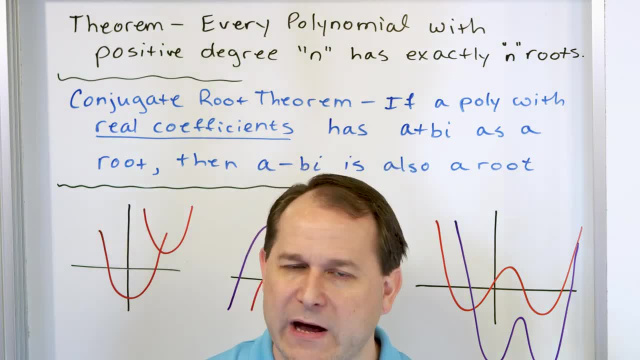 other two would be imaginary or complex roots, But either way, a fourth degree polynomial is still going to give you four roots. So just to wrap it up in a bow, this would be like an x squared. I'm not saying this is a graph of x squared. I'm saying this is a. 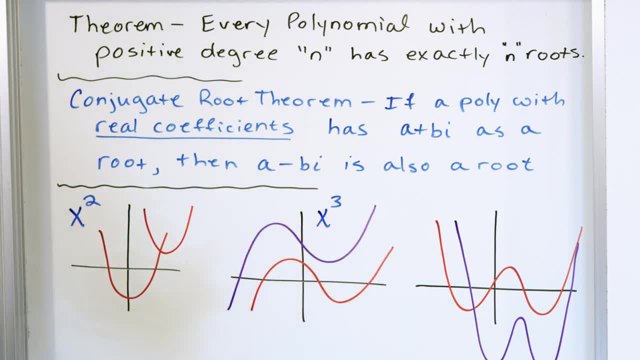 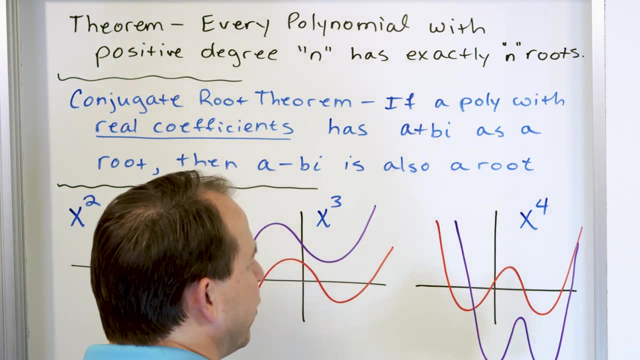 second degree polynomial. This would be like for a cubic type polynomial with all the terms after it. This would be for like a fourth degree polynomial. And again here you have in the red curve, you have the four real crossing points. Here's another example where you'd have two real and 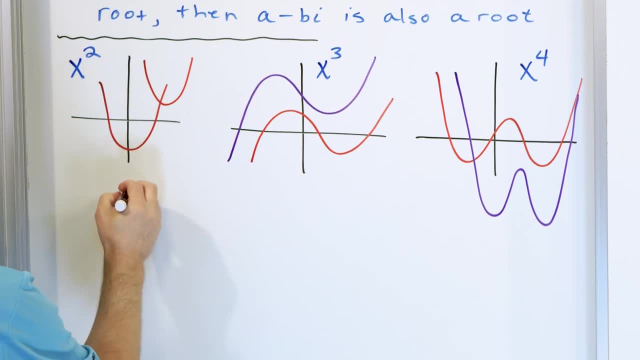 two imaginary crossing points. And then, of course, the first one, the fourth degree polynomial, would be a square polynomial. And then, of course, the first one that I opened up with was the concept of a line right And so for a line in general. 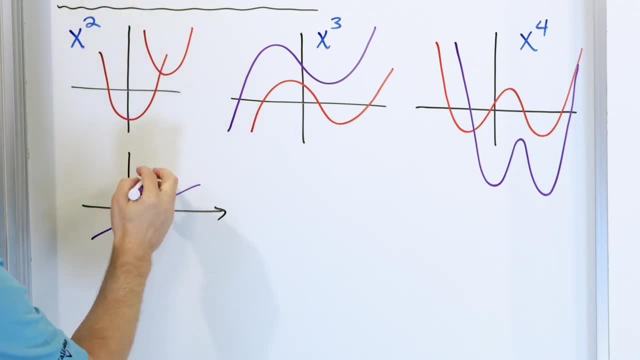 they can go either direction, but they're only going to have one crossing point, one root right here. So this would be like an x, y is equal to x type of deal. Of course that's not the exact curve, It's just generally a first degree, second degree, third degree, fourth degree, like this: 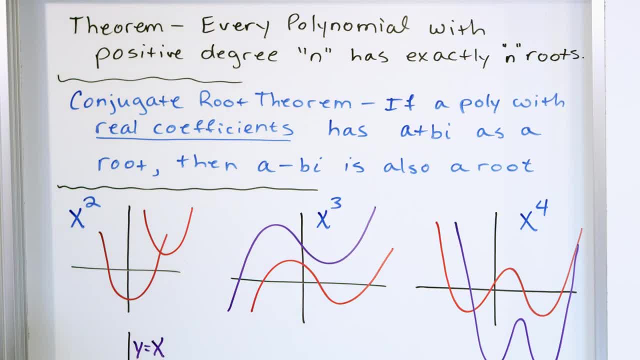 Now, the second theorem that I want to talk about is what we call the conjugate root theorem, And that is a theorem that you actually know also what it says. We've already talked about it, but we haven't formalized it. It's actually a theorem that I'll 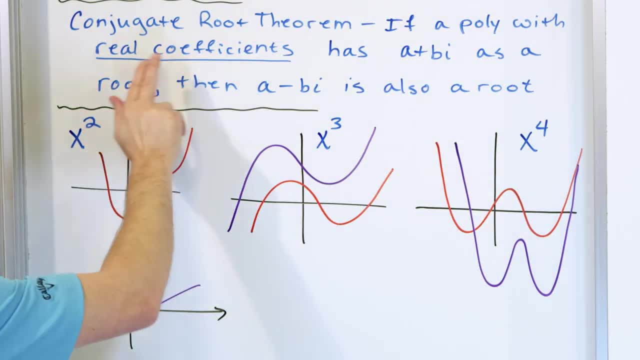 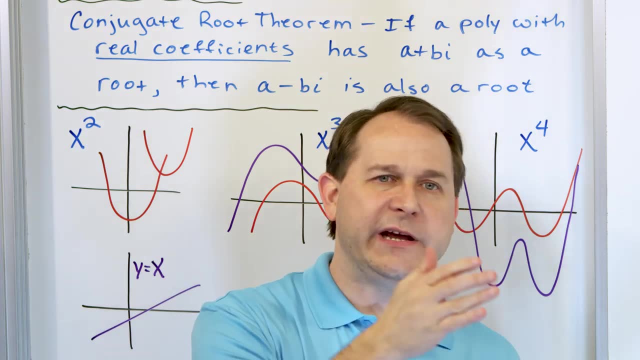 apply to all polynomials. But notice it says with real coefficients. Every polynomial we've ever done in this class has a real number as a coefficient in front of the x terms: right 3x squared, or minus 4x squared or something. Those are all real numbers. 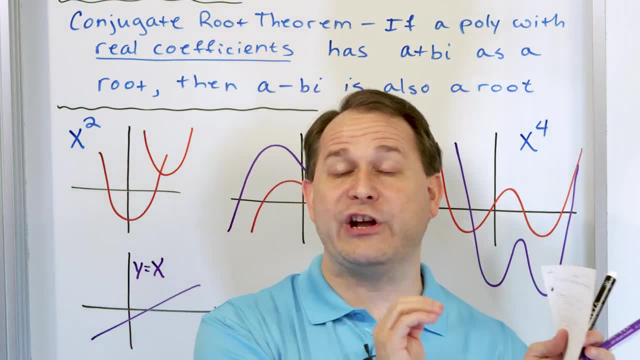 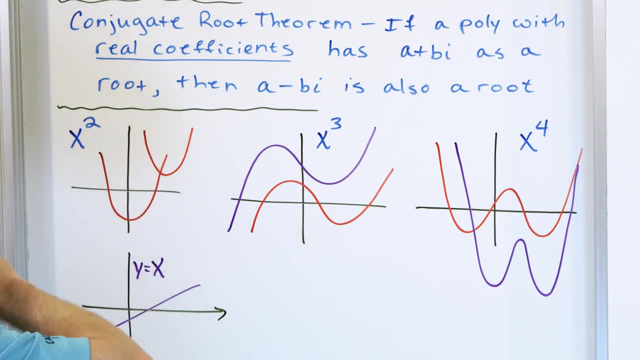 If you have a polynomial- and you can have polynomials with imaginary coefficients- then this conjugate root theorem doesn't apply. But for every polynomial we have ever dealt with, they always have real coefficients And what it's saying is: if you have an imaginary or complex, 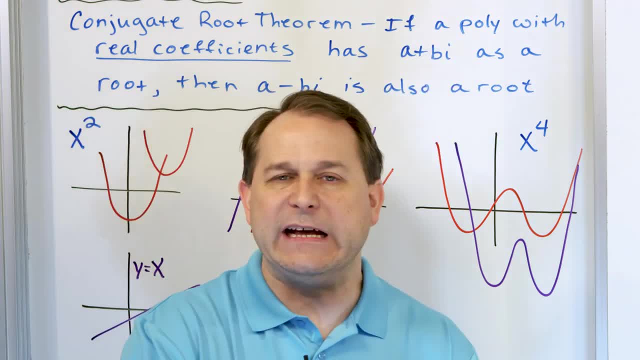 root a plus b, you're going to have an imaginary root. And if you have an imaginary root- a plus bi is just a general way of saying any complex number like 3 plus 4i- then if you know this root, 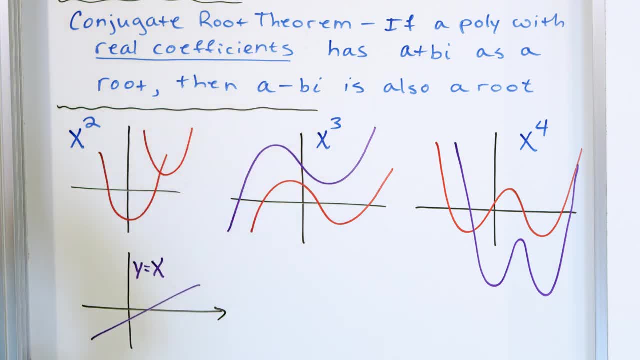 then you know that the partner root is called the conjugate root, which would be where the imaginary part has the opposite sign, And you know that that's going to be a root as well. So, for instance, if you know that 3 plus 2i is a root of a polynomial, 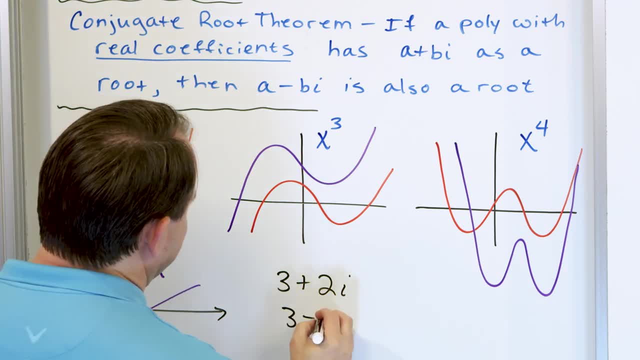 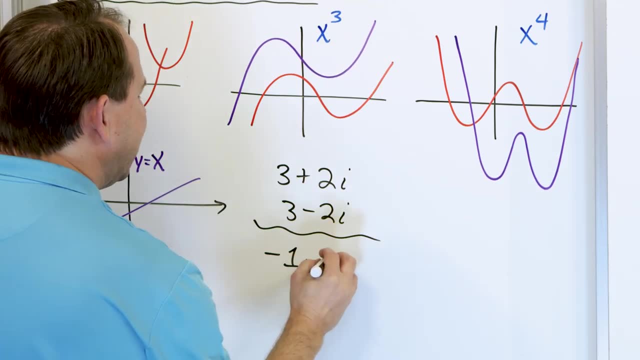 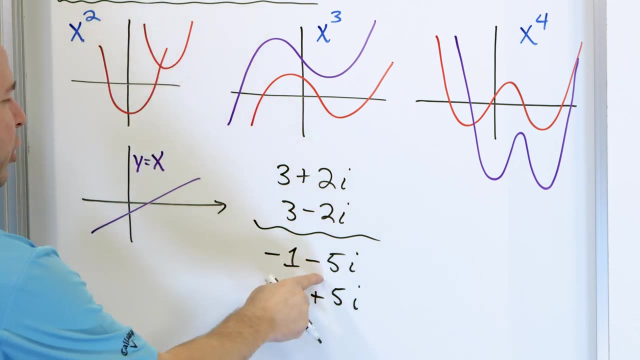 then by the conjugate root theorem you automatically know that 3 minus 2i is also a root. Right, And it goes the other way. If you know that negative 1 minus 5i is a root, then you automatically know that negative 1 plus 5i is also a root. These are called conjugate pairs. 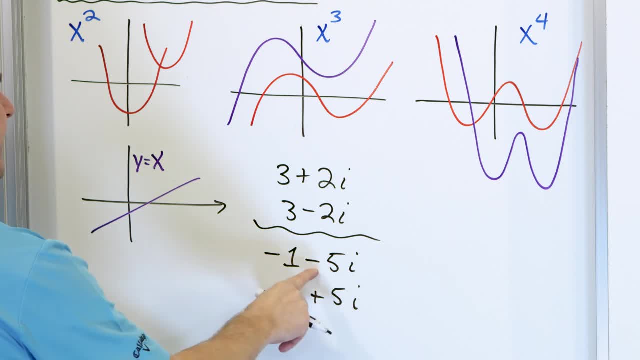 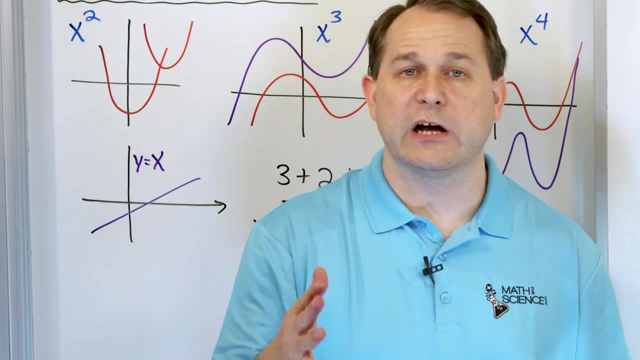 The only difference between them is the imaginary part has the opposite sign. Everything else is exactly the same. See the opposite sign here, opposite sign here. So the bottom line is: roots of equations. when it comes to the complex roots, they all 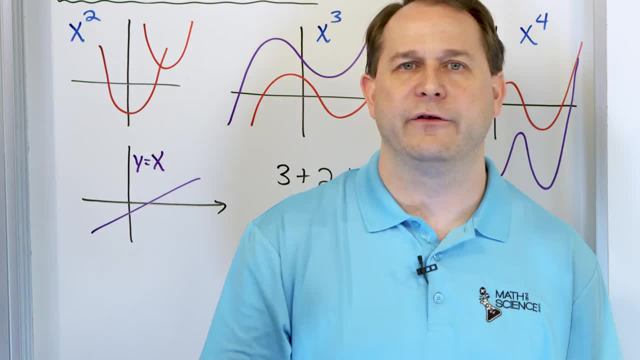 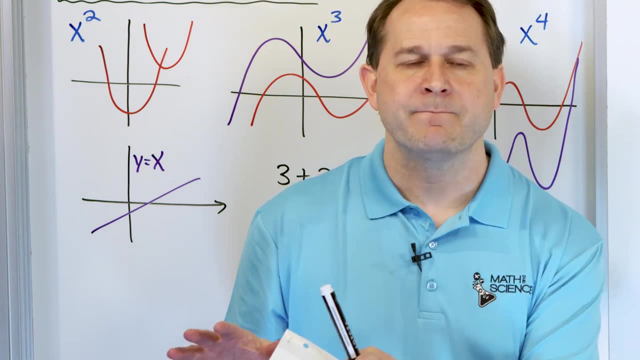 always come in pairs. You'll never, ever, ever, ever solve a polynomial equation and get a root that's complex without also getting the partner root, the conjugate of it. It's just always going to happen Unless this polynomial that you're dealing with does not even have real coefficients. 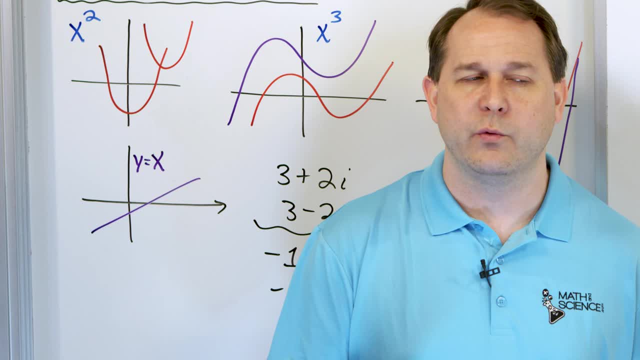 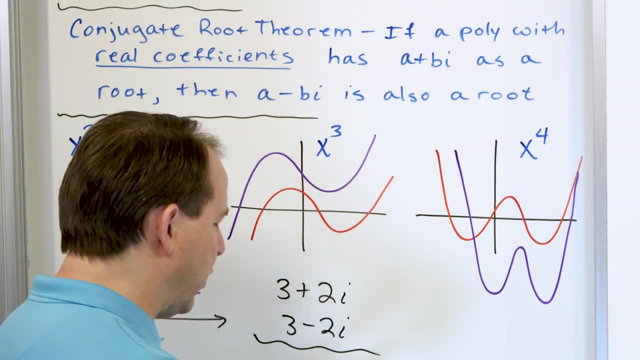 If it has complex coefficients or imaginary coefficients which we've actually never dealt with. but if you had that, then of course this theorem doesn't apply. But for every problem in this class, we're going to basically put our hats on this, because it's always going to be true. 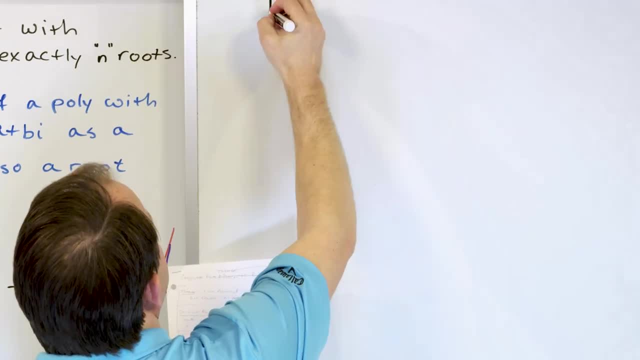 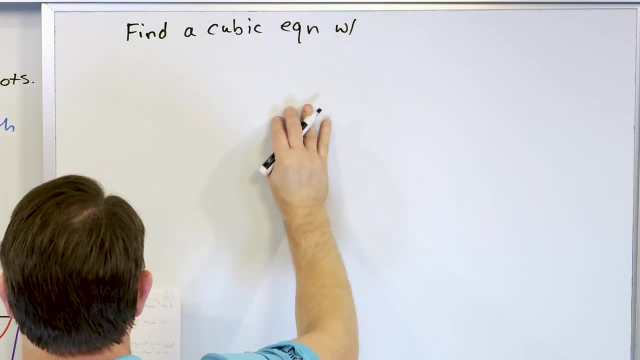 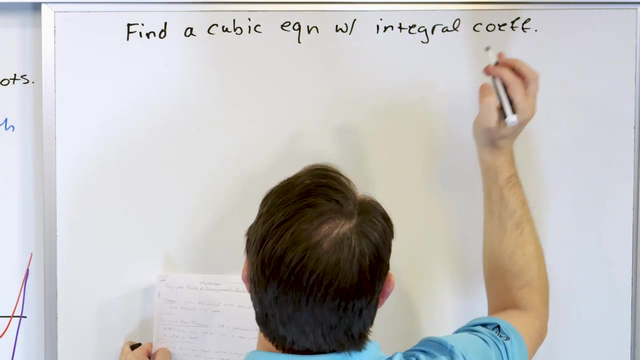 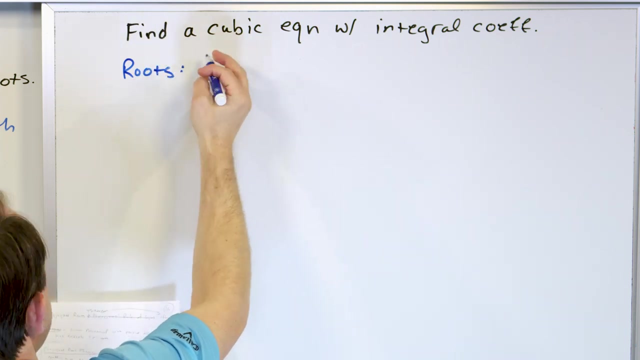 So the types of problems we're going to do here is the following. For instance, find a cubic equation with integral coefficients. Integral coefficients with the following roots: So the root for this problem is negative, 1 and 5i. Now I want you to find the cubic equation. 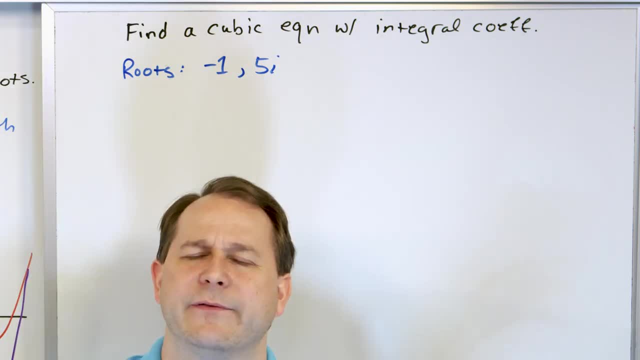 Now you might look at this and say, well, didn't we do this kind of problem before? Didn't he already give me the roots and then I had to find the equation. That's not the case. True, I did, But that was different, because, if you look here, I'm asking you to find a 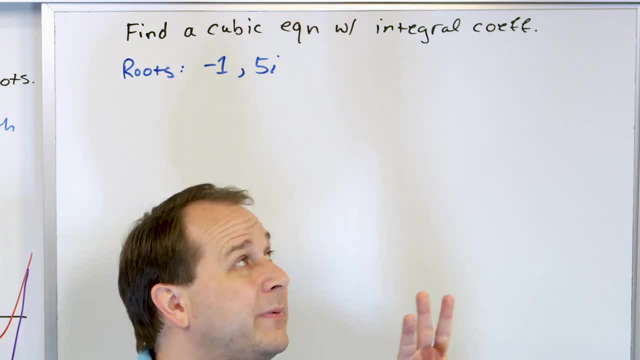 cubic equation That means a third degree polynomial. But I only gave you two roots, So you need to then know from the conjugate root theorem what the other root is. There's no way to really figure it out without knowing what the other root is, And because you know. 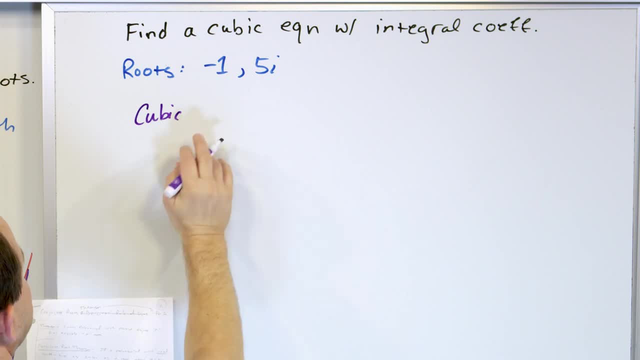 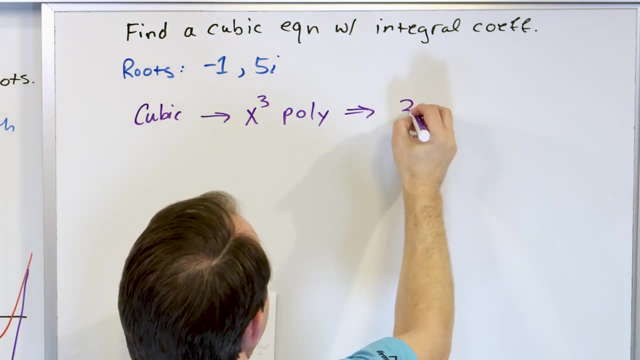 that it's a cubic. that's what we're asked to find. then you know that it's an x to the third power polynomial. That's what that tells you, right? And because of that, you know that there are going to be three roots. because of the first theorem that we already learned And you already. 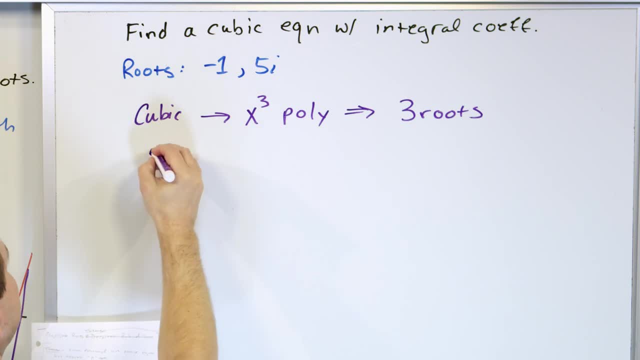 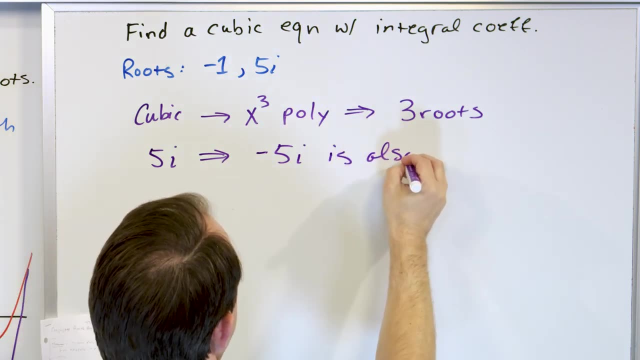 know what two of them are and one of them is imaginary. So that means that the 5i root produces a partner root which is negative. 5i is also a root right Now, if you look at the wording here. 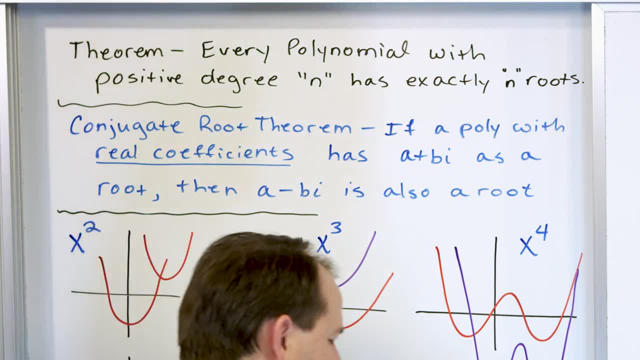 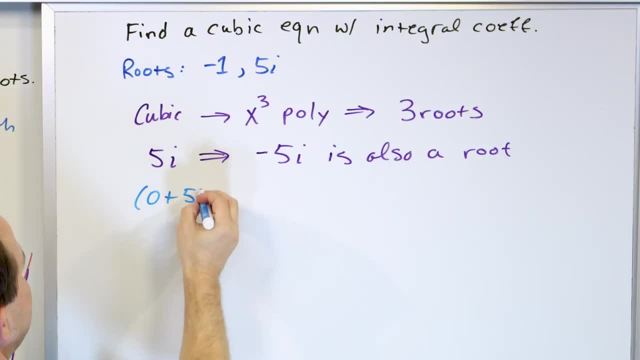 it says a plus bi and then a minus bi are also roots. So another way of thinking about it is: if you know that one of the roots is 5i, that's basically the complex number 0 plus 5i, That's. 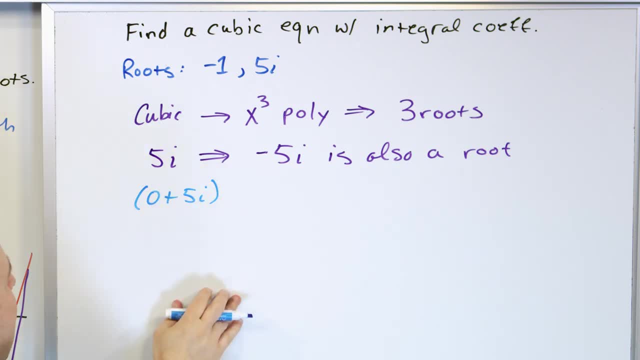 what that means. No real part at all, but the imaginary part's 5i, And that means the conjugate of it is 0 minus 5i, And if you just strip the 0 away, then this is what I wrote down here. So 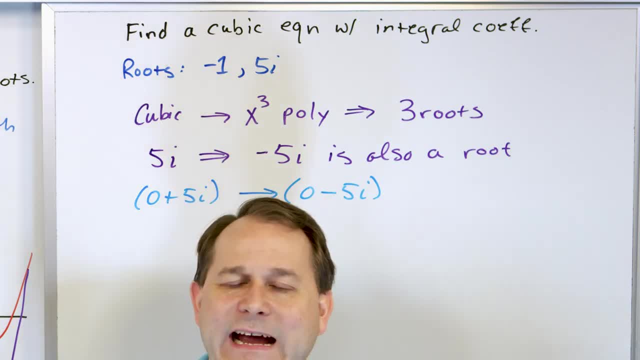 for conjugate numbers. if it's purely imaginary, you just stick a negative sign on the front, Or if it was already negative, you flip it back to positive. If it's complex, then you just retain the real part and flip the imaginary part. So it's all the same thing. But the bottom line is: 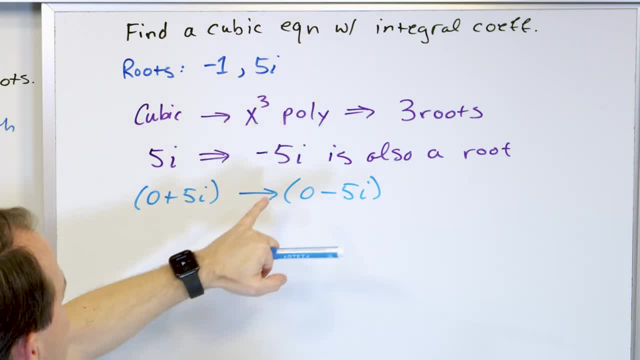 we now know that since 5i is a root, then we know that negative 5i is a positive root, So we know that negative 5i is also a root, And that's because of this conjugate root theorem, And so 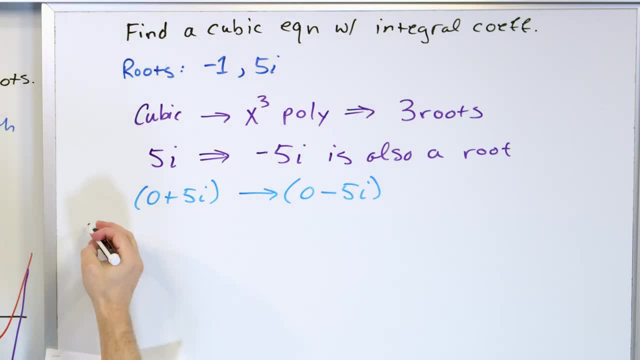 since you now know what all three roots are, you can construct the polynomial the same way we did before. For this root, it will be x plus 1, because the factor will be x minus a negative 1.. We've done that many times before. And then for this root, it's going to be x minus 5i. 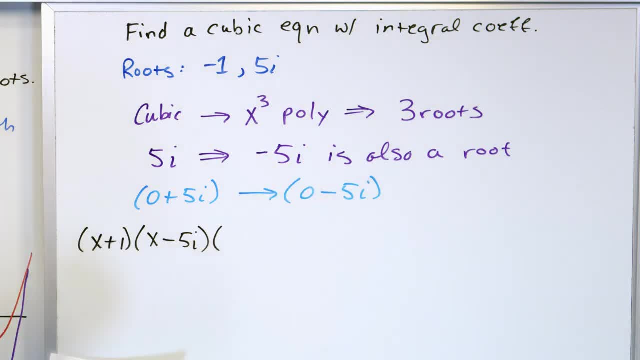 And then for the root that we now know is additional from the conjugate root theorem, it has to be x plus 5i And that has to equal 0.. And if you think about it, if I give you this and I ask you what are the roots of this equation, you set this equal to 0,. 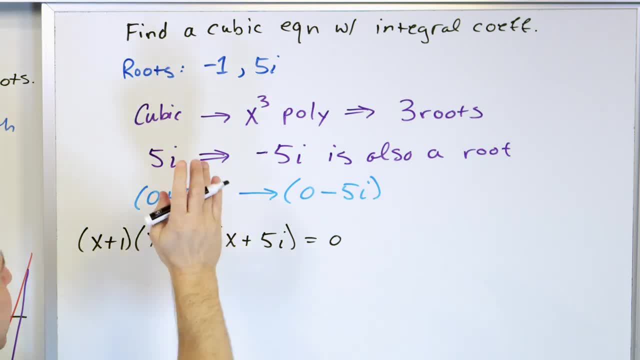 solve for x: you get negative 1.. Set this to 0, move this over: you get 5i. Set this to 0, move it over: you get the negative 5i. So you know that these factors have been correct. 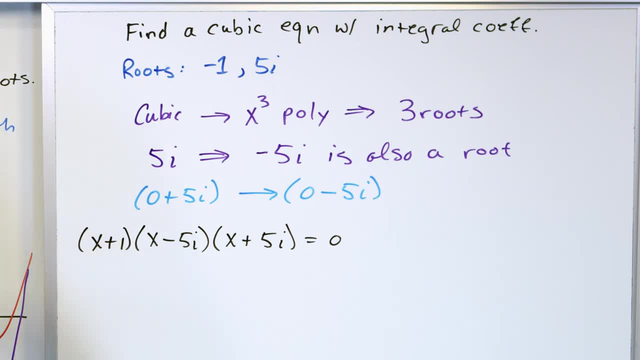 Now what we have to do is perform the multiplication to figure out what the parent polynomial is. You have to multiply this out, So we'll save the x plus 1 for last And we'll multiply this x times. x is x squared. This is going to be: 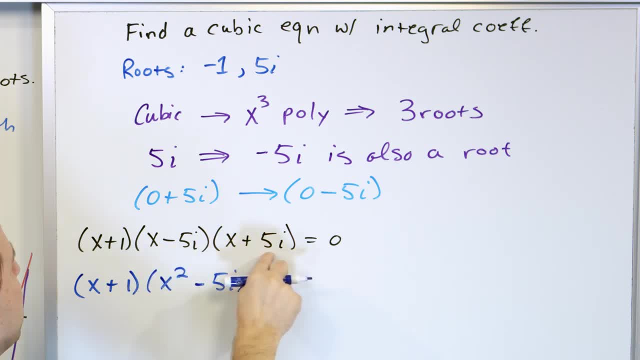 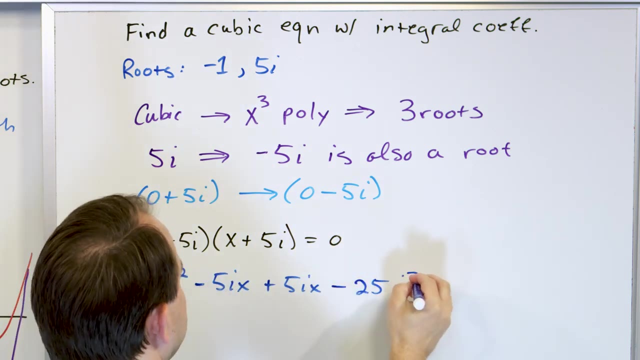 negative 5i x, Then this one will be positive 5i x. okay, We multiply them with these guys here: Negative 5i, positive 5i, we'll give you a negative because the negative times a positive 25, and then the i times the i is, i squared, Easy to make. 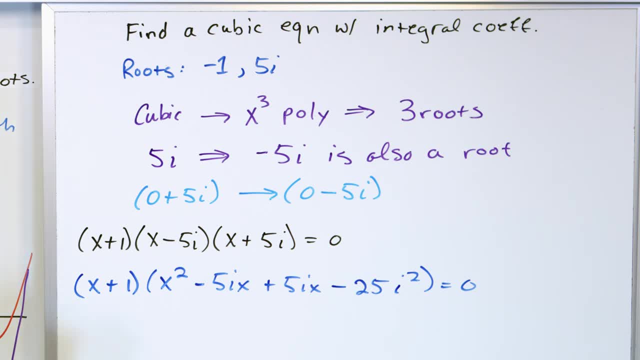 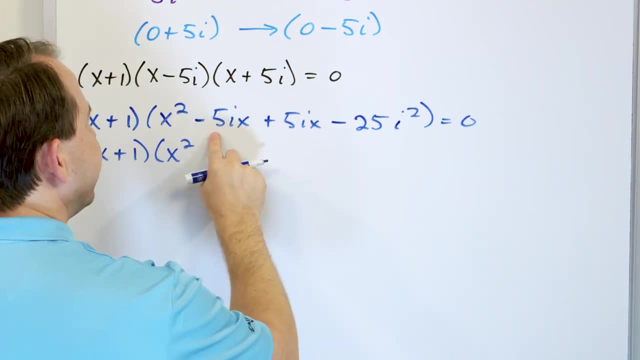 mistakes with complex numbers and imaginary numbers like that. so we have to know how to deal with that. And then on the next line we'll say: well, we'll take the x squared term and we'll add these together, but these add to 0.. Negative 5i x. 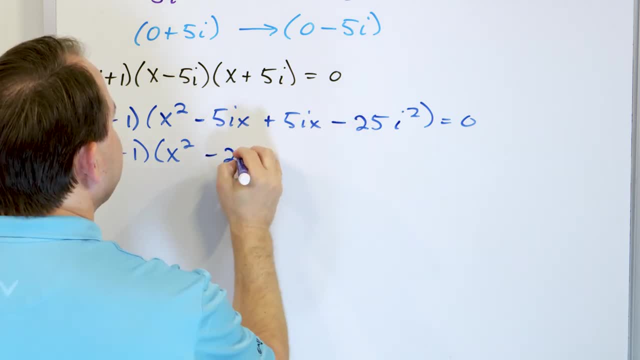 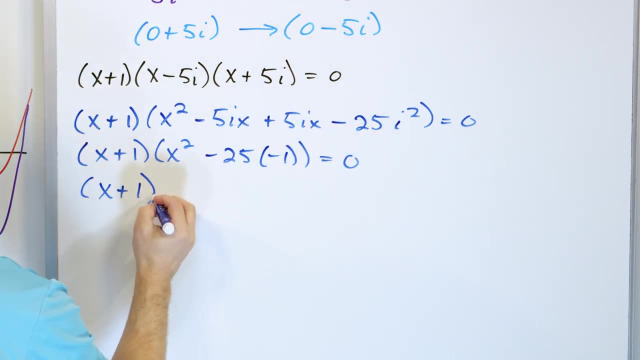 positive i by x, And then this is negative 25. But then I know that i squared is negative 1. So I'm going to write it like this, And in the next line I will simplify it to kind of its final form. 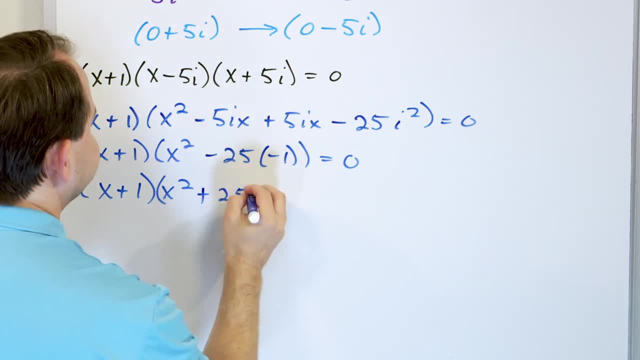 x squared, this becomes plus 25.. All right, So far, so good. So the way I want to do this, when you have very complex multiplication, is just multiply two of them. When you get the answer, multiply that by the next one. 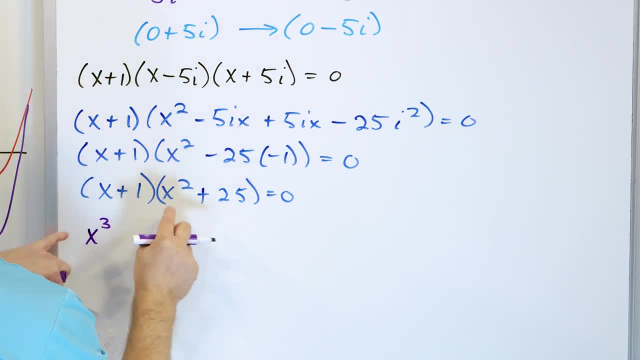 So then you have to multiply: x times x squared is x cubed. Then x times the 25 is 25x. Then 1 times x squared is x squared 1 times 25 is 25.. And now we collect terms. 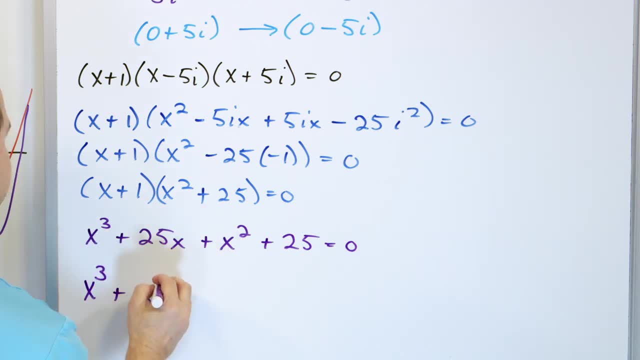 We have x cubed. This x squared is the next lowest term, And then the 25x, And then the 25.. And you circle this. So x cubed plus x squared plus 25x plus 25 is equal to 0.. 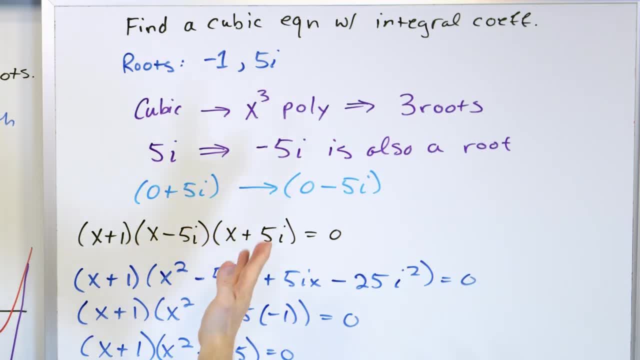 And if you were to plot this, we know already that 2x squared plus x squared plus 25x plus 25 is equal to 0.. One of the roots is purely real. It's a real root, But two of these roots are complex. 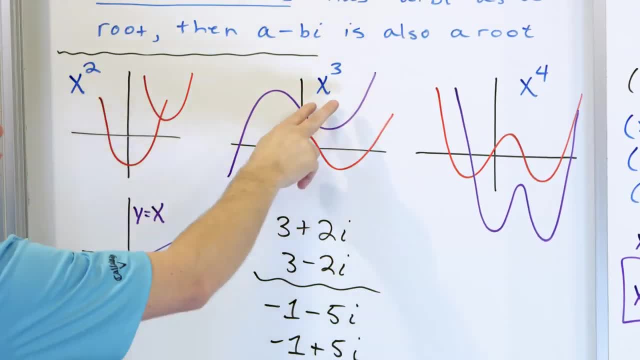 They're conjugates of one another. So, going back to our original sketches, we know in general that cubics are going to look like this. They're going to look like a little s that goes down, But in this case it might look more like the purple curve. 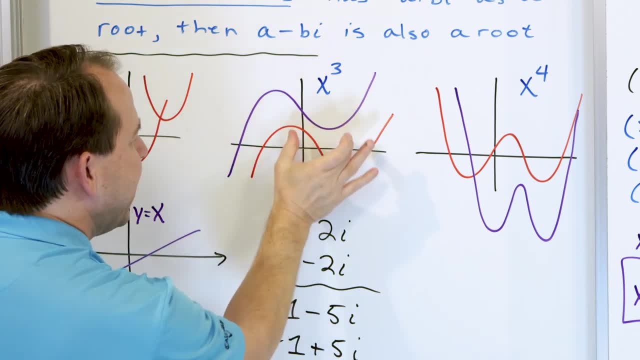 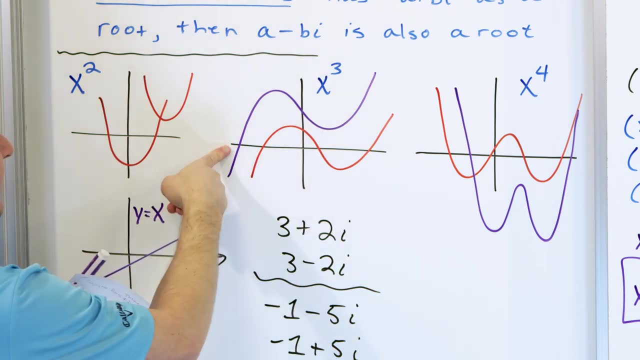 where you have one real crossing point and then the other two never really made it down to cross. So they're representing the imaginary, the complex roots. So if you rescale it this would be like at negative 1.. That's the real root here. 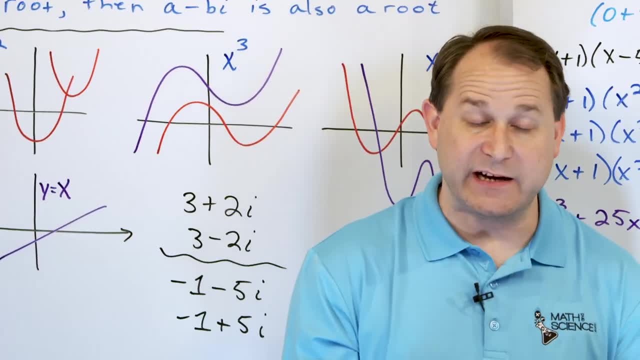 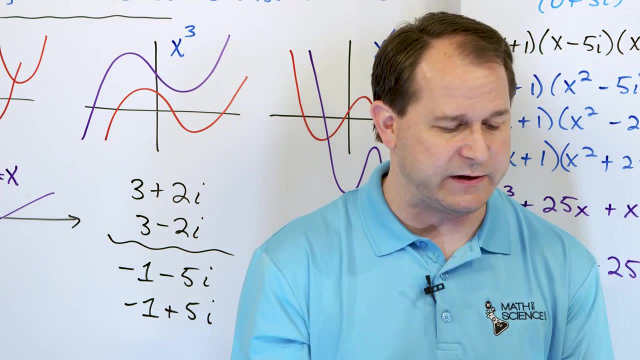 These represent the plus and minus Minus 5i, And I've done an entire lesson on what do complex and imaginary roots mean. So if you want to see more information about that, you can go dig up that lesson that I've done. 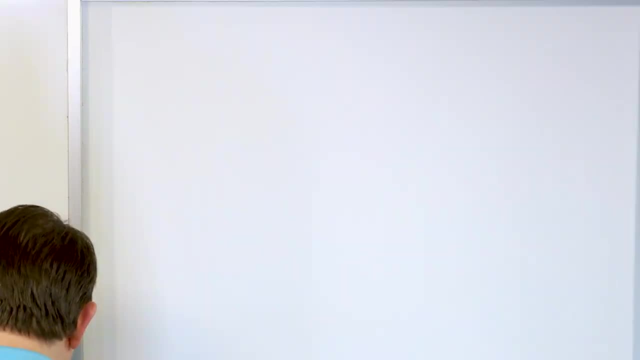 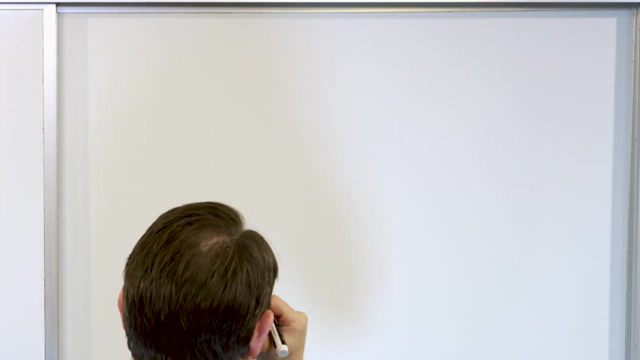 So this, basically, is very similar to the previous problems we've done, but we're just using the conjugate root theorem and the number of roots that we know now as a theorem as well. So we also want to find a cubic with integral coefficients. 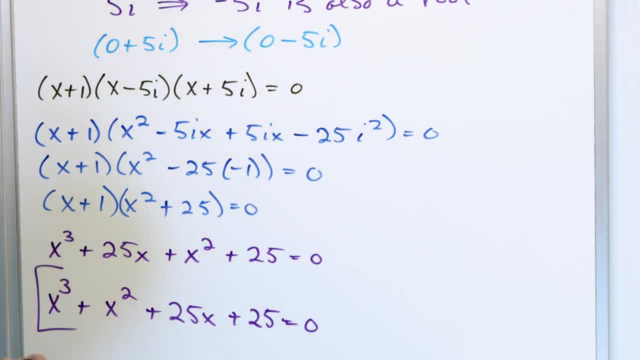 Notice, we have integral coefficients. That's the other thing we know. And then I want to say one more thing before I move on. I mentioned it in previous lessons. This equation does have these three roots that we've talked about, But it is not the only equation that has those roots. 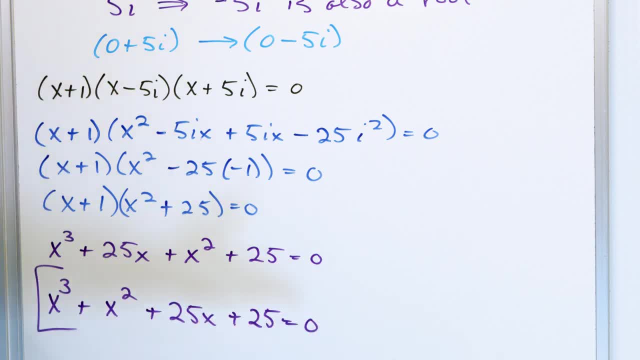 If I multiply the left-hand side and the right-hand side by any number I want, let's say I multiply by 5, then I'll get 5x cubed plus 5x squared, plus 125x plus 125. I'll get a much higher coefficients, right? 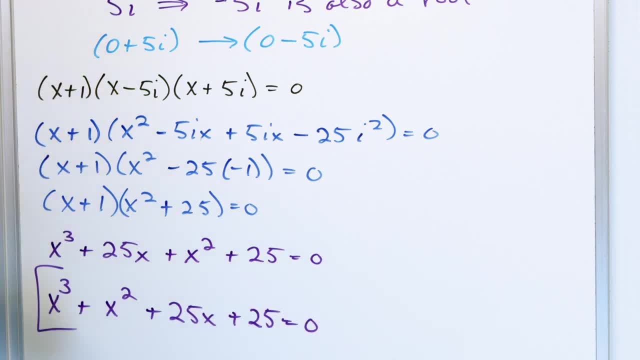 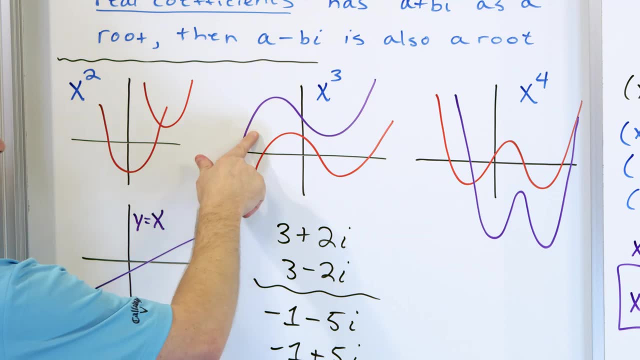 Yeah, Equals 0, because 5 times 0 on the right is still going to be 0. Then I will get a different polynomial that will graph differently than this one. let's say, Maybe it goes much higher, and so on and so forth. 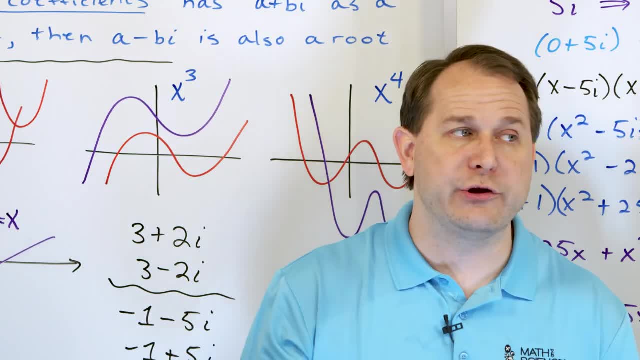 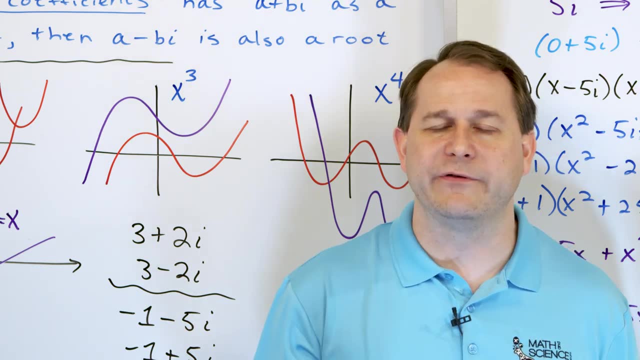 but it will still have the same roots, right? So you can take the answers you get here. You can multiply them by anything you want to generate another polynomial. That new polynomial will have the same roots as the one this one has, but it will be shaped differently. 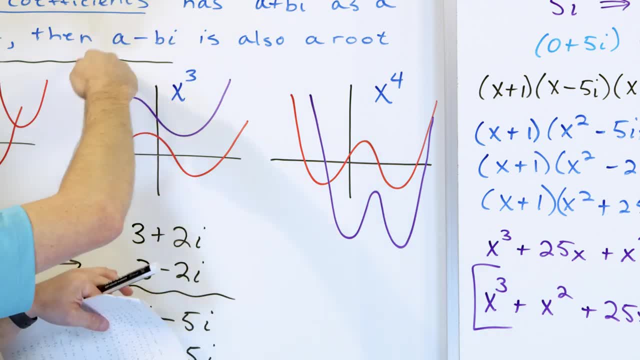 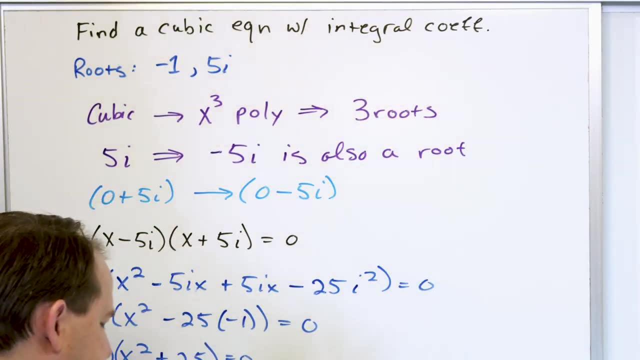 So if I multiply any of these curves by a number, I might stretch the curve, But they'll still have the same crossing points there. So the reason I bring it up is because this is saying: find a cubic with integral coefficients, In this case the polynomial I already arrived at. 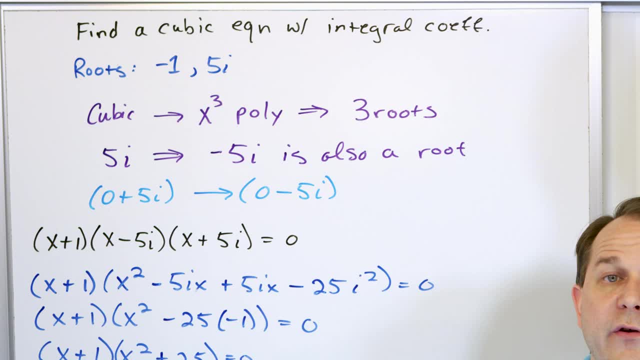 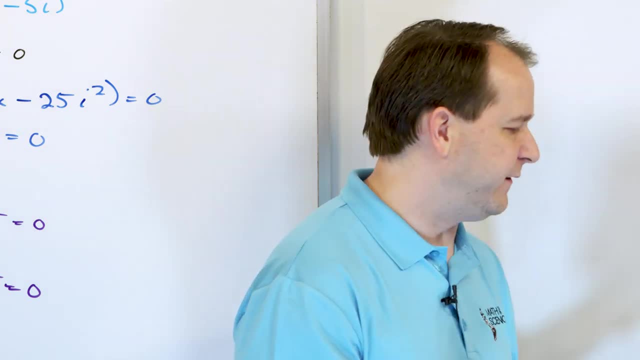 already had integral coefficients- no fractions, in other words- So I didn't have to mess around with it. But if I needed to multiply that polynomial by 2,, I could do that, or by 5, or by whatever I wanted to. 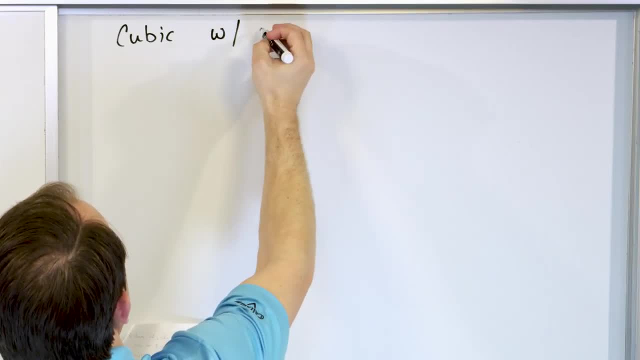 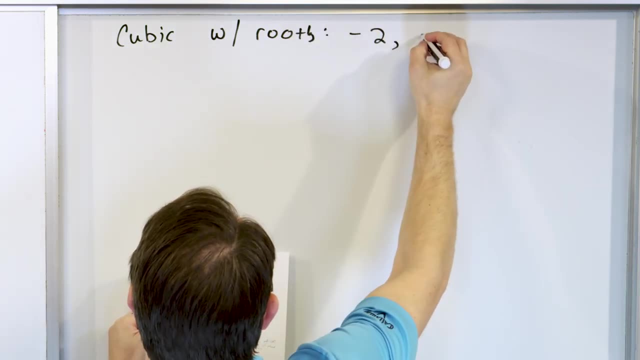 So here I'm still trying to find a cubic, And here I have roots that are given to me, if I can spell the word, roots of negative 2.. And the other root is negative 1 plus i. So again, I'm told ahead of time as part of this problem. 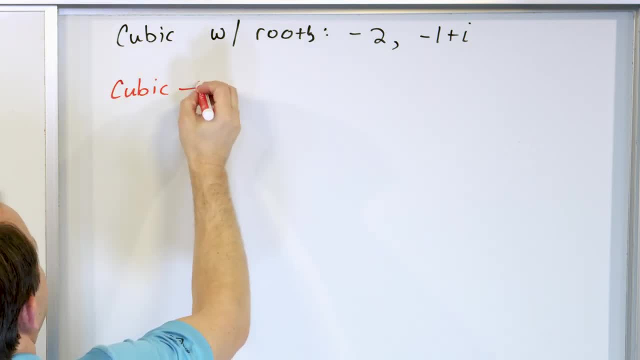 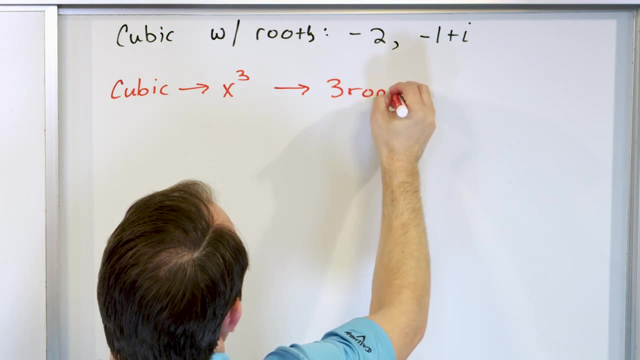 that I want a cubic right, And so, because I want a cubic, I know that I want a polynomial with a third degree highest power, which means I need three roots. But I've only been given two of the roots, and one of them was real, one of them was complex. 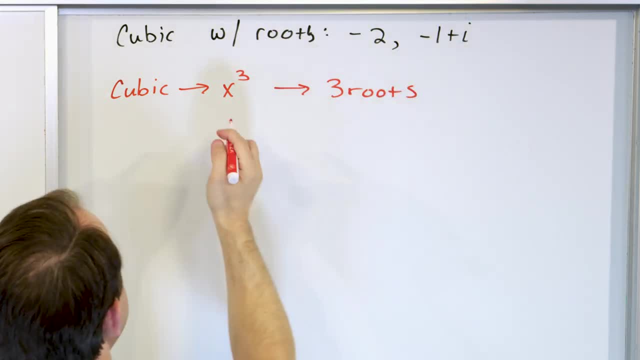 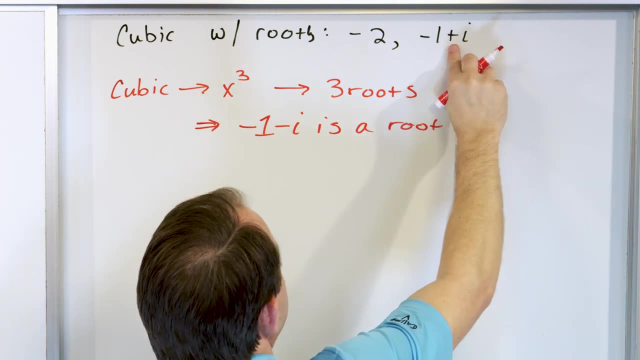 And because I know all of the complex roots come in pairs, then I must also then have negative 1 minus i is a root. Because this is a complex root, I know that the conjugate of it must also be a root. This would be one, two, three roots. 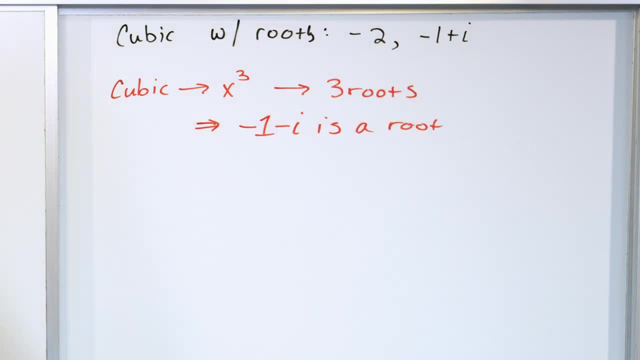 altogether for my cubic that I'm trying to find. So then, in order to actually find it, I have to write the factored form. This root is going to lead to a term x plus 2.. This term is going to lead to, because it's basically: 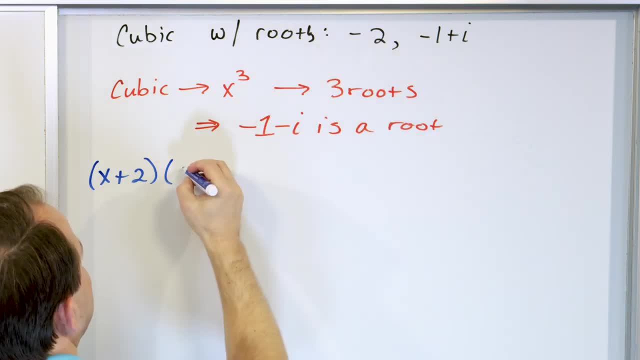 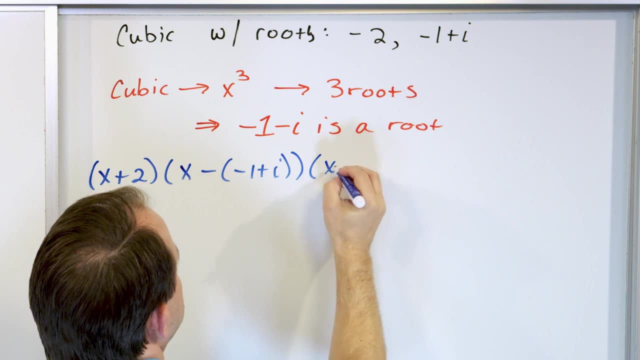 x minus the minus 2.. That's why it's x plus 2.. This one is going to become this is how you write it down: x minus negative, 1 plus i. And then this last one here will be x minus negative, 1 minus i. 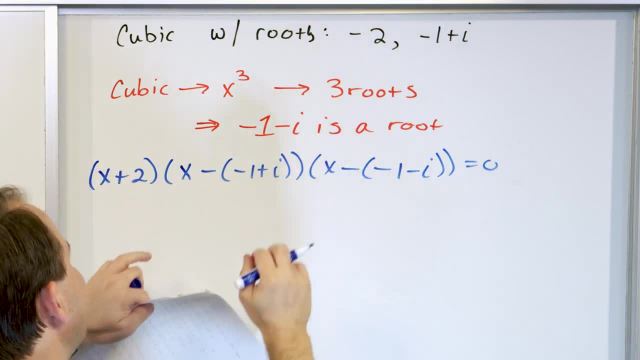 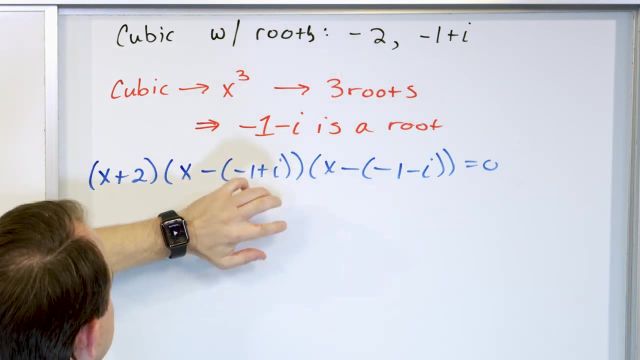 Now, the reason these are written this way is because if I were to give you this and say what are the roots, what would you do? You would set this to 0 and solve it and find that that's negative 2. You would set this one to 0.. 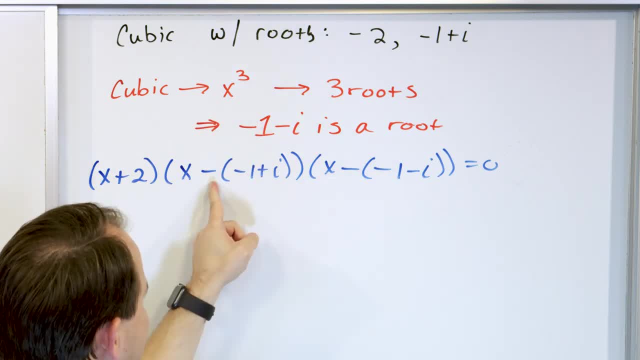 You would take this whole imaginary complex term, move it to the other side by addition and you would find that negative 1 plus i is a root. And then you would do the same thing here and you would find this is a root. 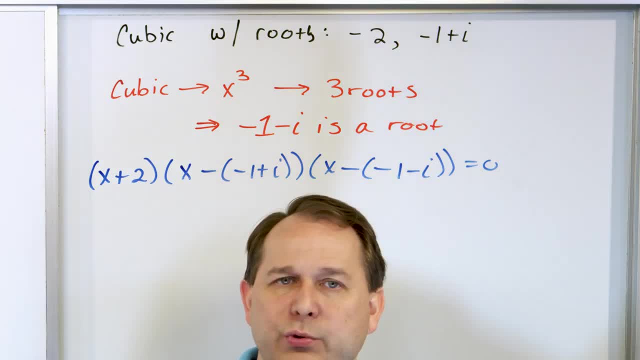 So the bottom line is: whatever root you're given, you just say x minus that root. That is one of the factors and that comes from the factor theorem that we've already learned. So now that that's out of the way, we have to multiply all this stuff out. 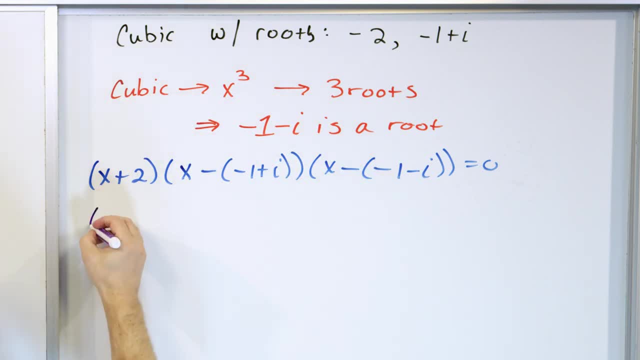 But before we can multiply we have to fix what's on the inside here. So we have x plus 2. And this becomes x minus times. minus gives us positive 1.. Negative times i is negative i. And then we have x minus times. minus is positive 1.. 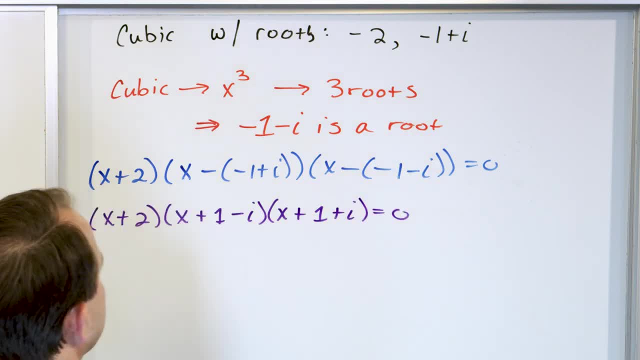 Minus times minus is positive i. So now we have two very large, complex terms, and then we have another one here. So what we want to do is multiply only these two terms together first. Whatever we get as an answer, we'll then. 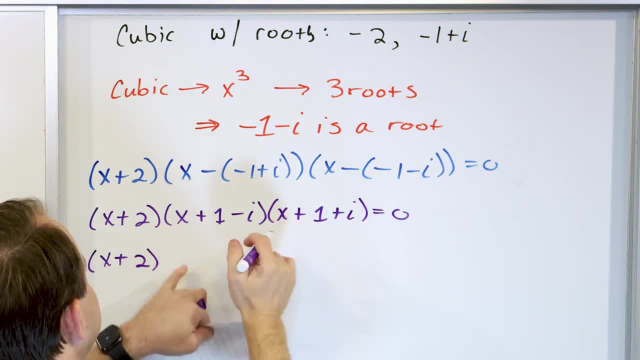 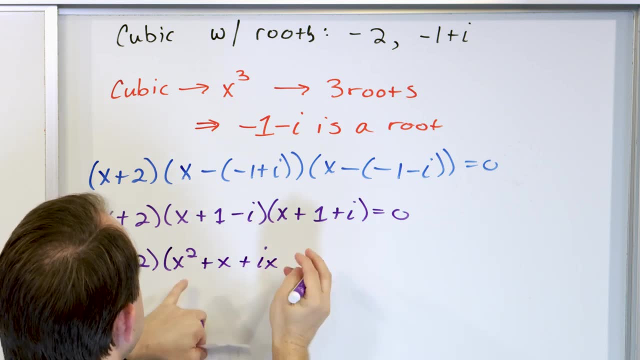 multiply by the x plus 2 there. So x times x gives me x. squared: x times 1 is x, x times i is i times x. Then I move my finger here: 1 times x is x. 1 times 1 is 1.. 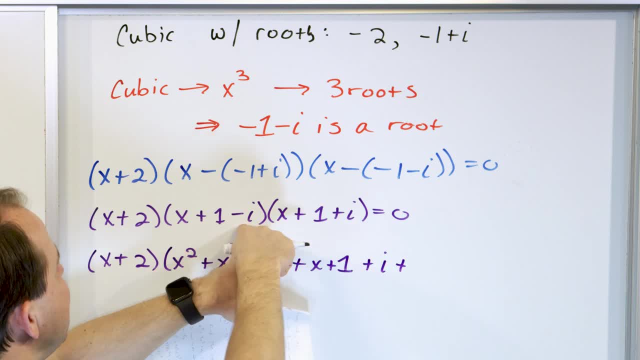 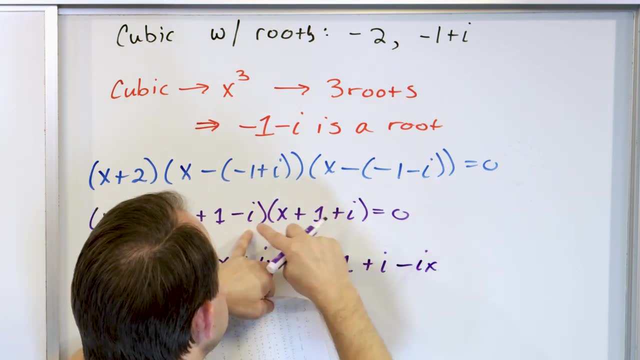 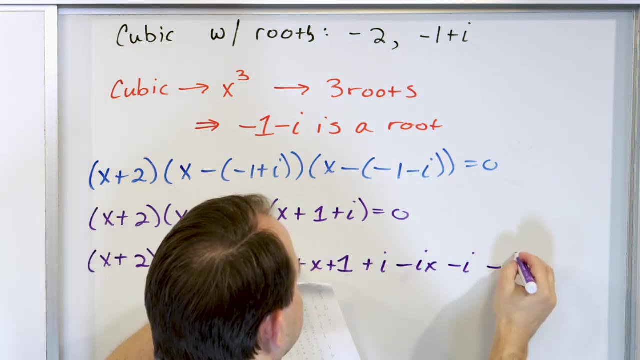 1 times i is i- I move my finger here- Negative i times x is negative. i times x is negative. ix Negative i times 1 is negative i Negative i times i is- don't forget, be careful. negative i squared. 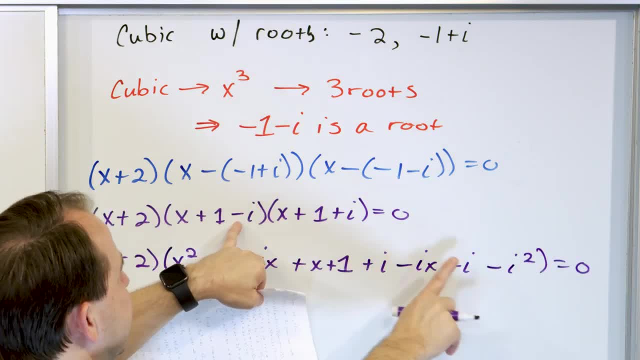 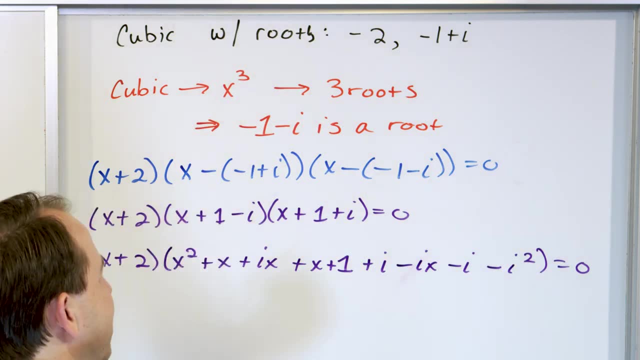 Do not try to do too many things at a time. The negative times, positive means I have a negative sign. The i times the i gives me i squared. Yes, I know that. you know that this i squared will eventually become a negative 1.. 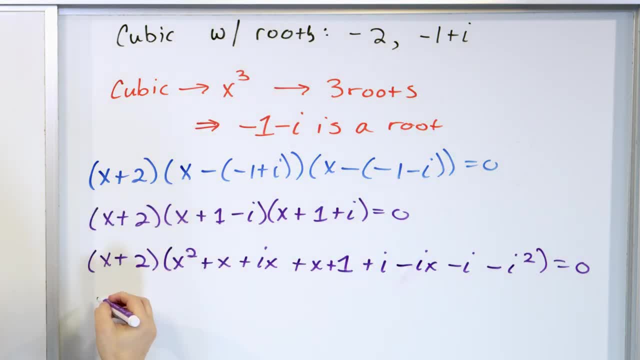 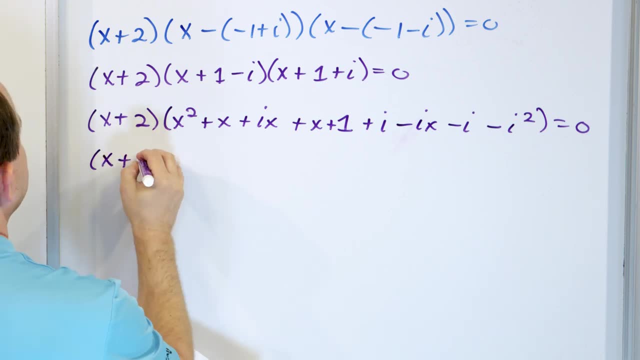 But to keep it clean, write it like that Enough, Initially. Then we're going to clean up our terms And I think the way I'm going to clean up my terms, Yeah, like this: x plus 2.. And on the inside here, 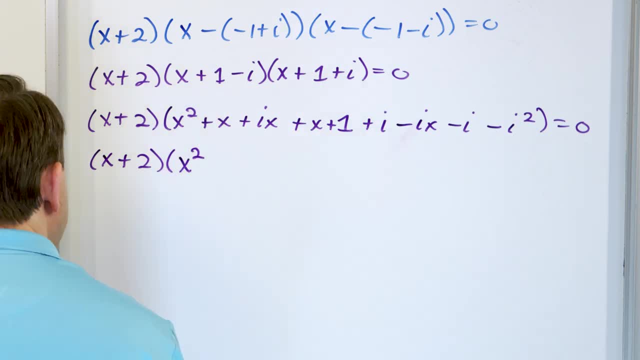 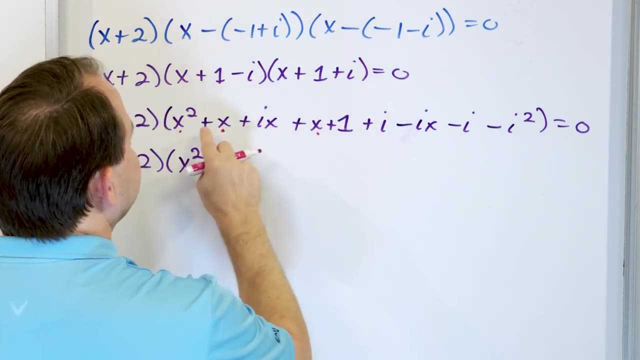 I look for x squared. I got an x squared term. I'm gonna put a little dot under that to tell me I've looked at it. I have an x term here and an x term here. X term here and x term here. 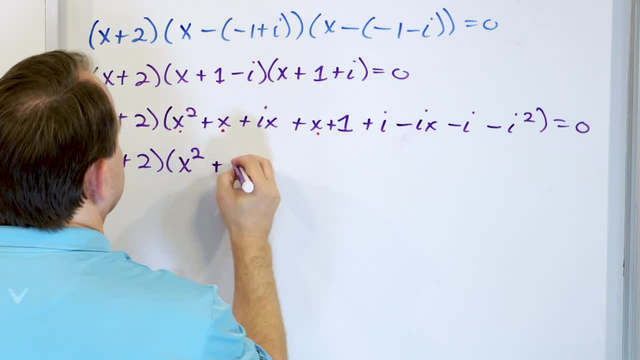 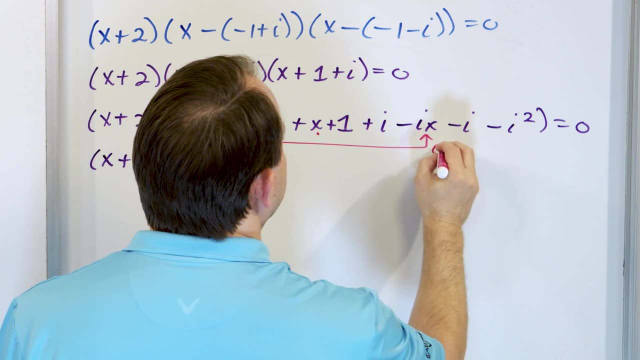 That's gonna be 2x All right, but then I have an ix term here and a negative ix term here. So what I'm gonna do? and a negative ix term here here, So these guys go together and basically add to zero. So I've taken care of this one. 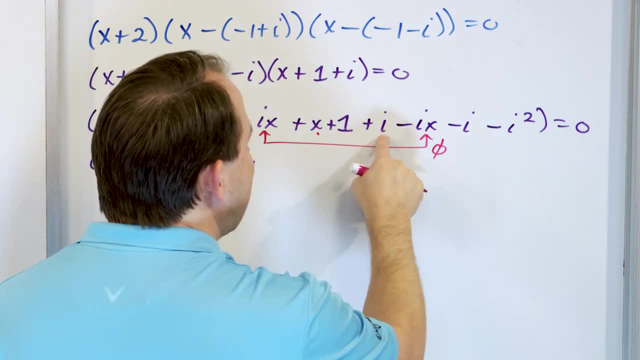 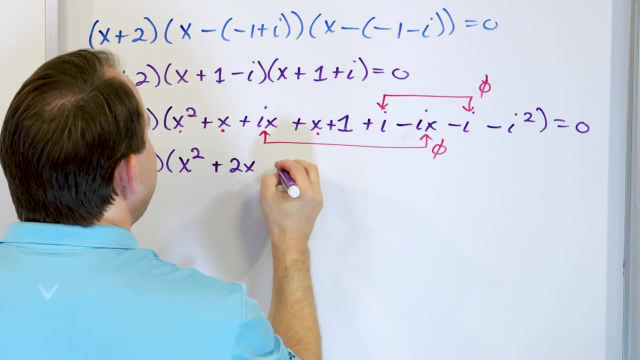 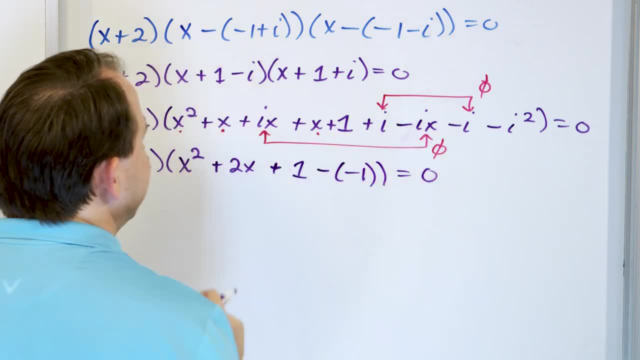 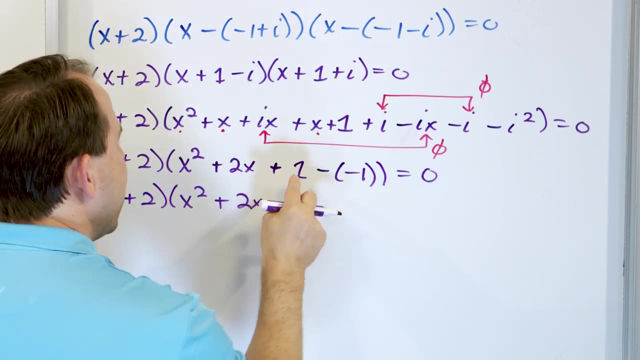 i squared is negative one. That's when you finally deal with that at the end And then it becomes very simple, because what you have is x squared plus two x, And then you have one. But this becomes a positive one. I'm sorry, Yeah, positive one. Negative times. negative is positive one plus. 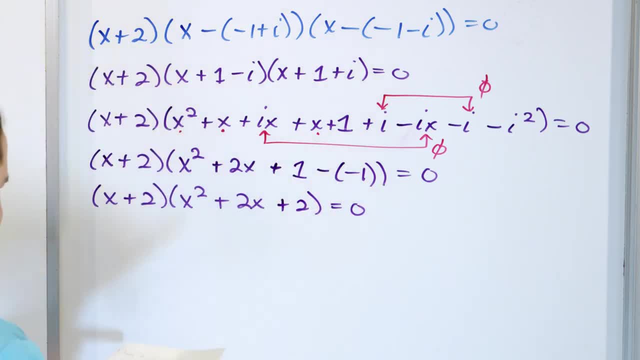 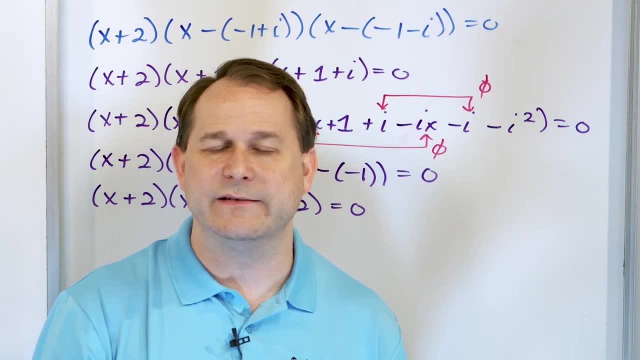 the one gives you two. So let me double check myself: I have x squared plus two, x plus two, And that's correct. It's very easy when you're multiplying complex numbers and imaginary numbers, to screw up the signs, Because if you're trying to do i squared is negative one and you have. 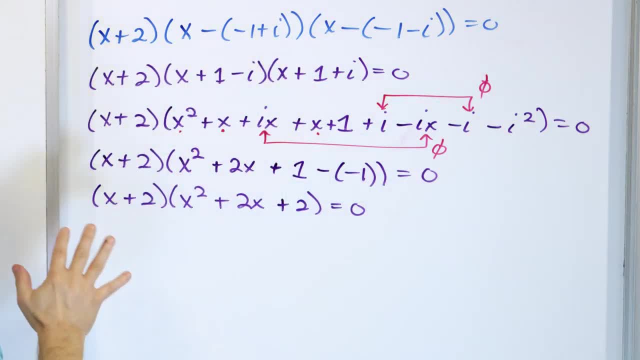 negative times negative and all that. it's very difficult to keep it straight And that's why I'm showing you how i tip. I typically do it All right. Next thing we need to do is multiply these together: x times x gives me x, I'm sorry. x times x squared gives us x. cubed x times the two x is two x squared. 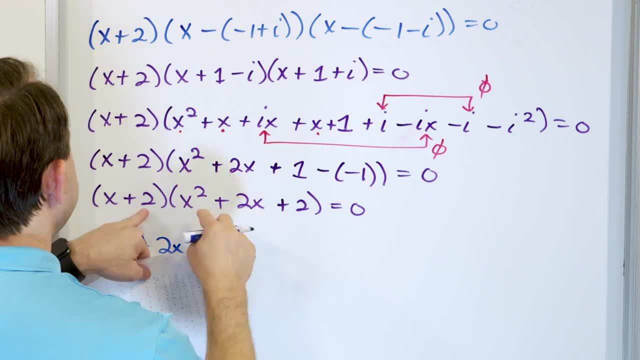 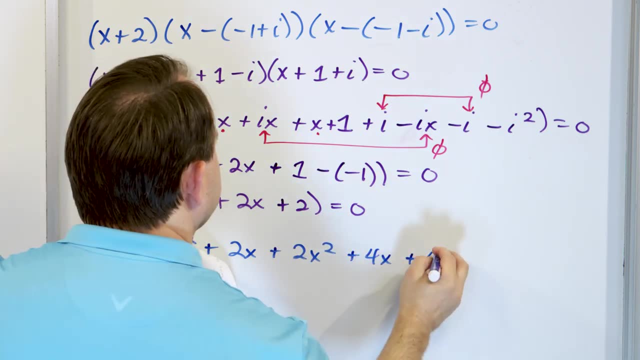 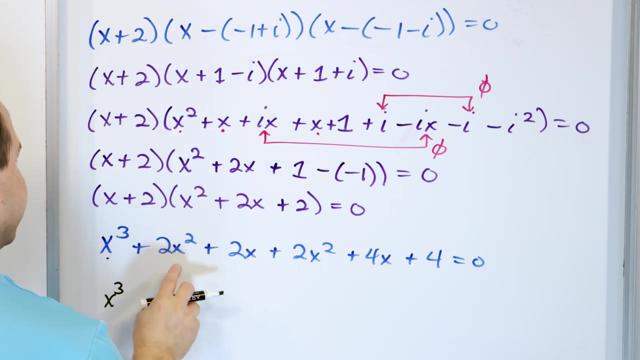 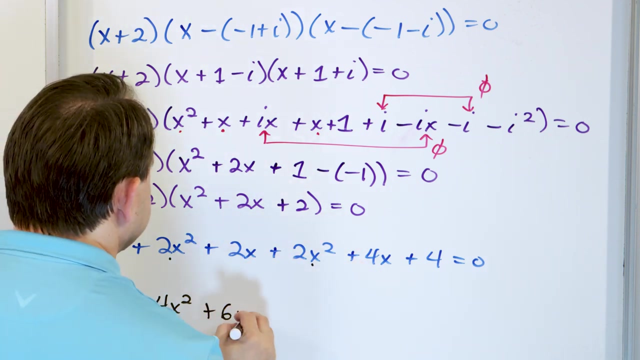 x times the two is two x, And then we have two x squared, And then we have four x, And then we have four, And then we collect terms again. All right, So we have x cubed, two x squared, that's a four x squared. Put a dot there and a dot there: Two x and a four x is six x, And then 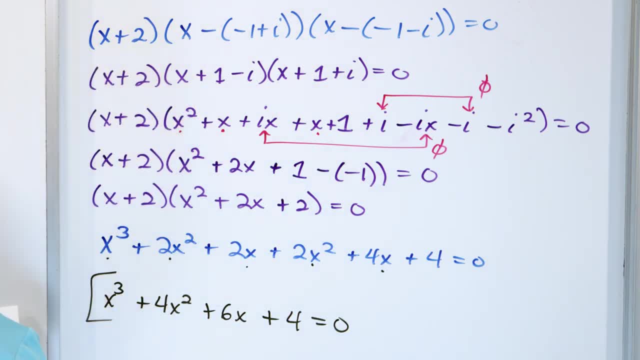 we have a four right here And I'll double check myself: x cubed plus four, x squared plus six, x plus four, that equals zero. And again we check because the problem said: find a cubic equation with integral coefficients. with these roots, All of the coefficients are basically there are no. 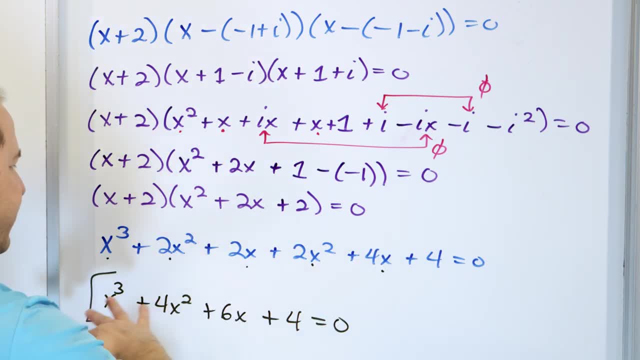 fractions. They're integral coefficients, So I don't need to multiply this equation by anything to clear out any fractions. I don't need to multiply this equation by anything to clear out any fractions. I've already have integral coefficients, so I'm good. But also keep in mind- this is just one of 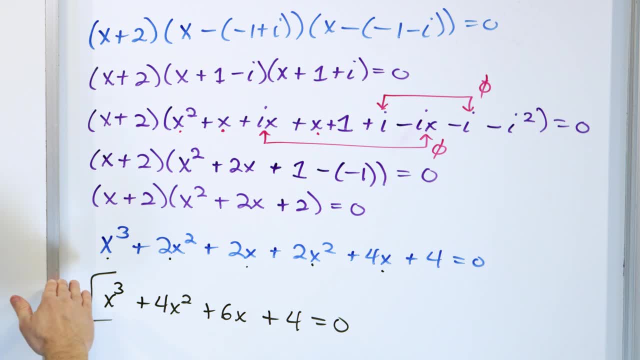 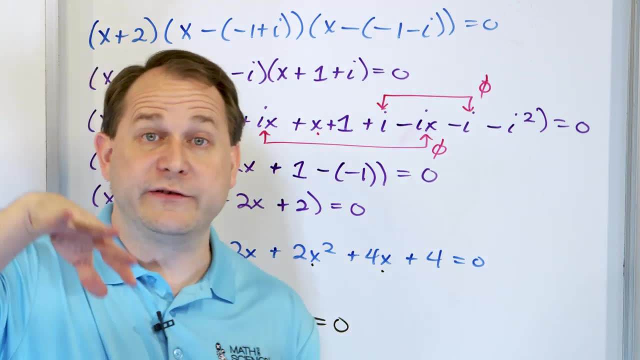 many equations and one of an infinite family that has the same roots. If I multiply this equation by four, or by five or by 10, I will get new coefficients. The curve will look different, but it will still cross in the same locations, So I will have. if I did that, I would have a. 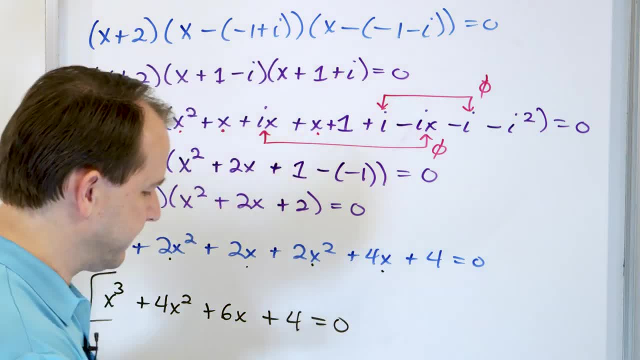 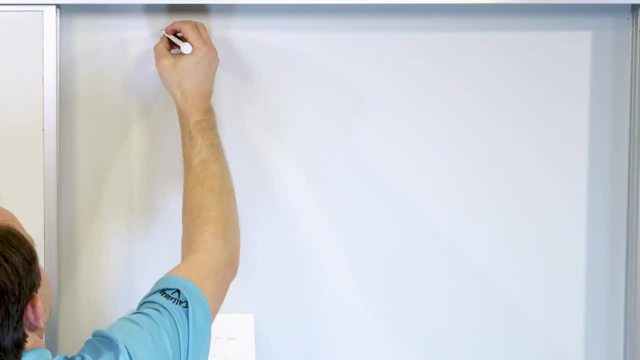 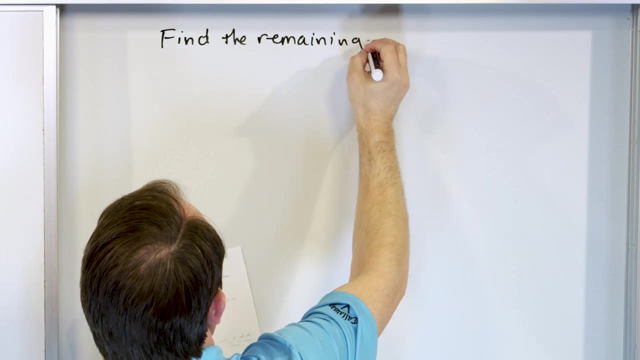 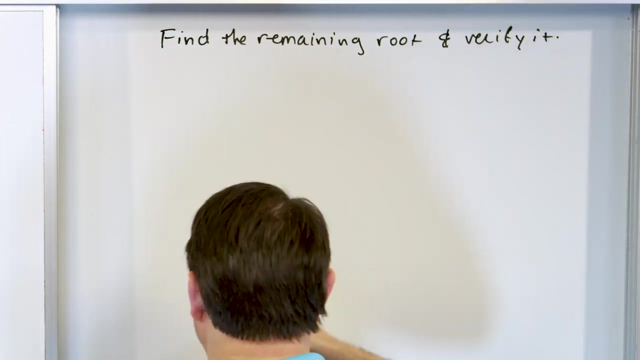 similar equation that's related to this, one that has the same roots. Okay, Last question. It says the following: Find the remaining root and verify, Verify it. So what I'm going to do is I'm going to give you some roots. You're going to have to figure out what root is left and go from there. 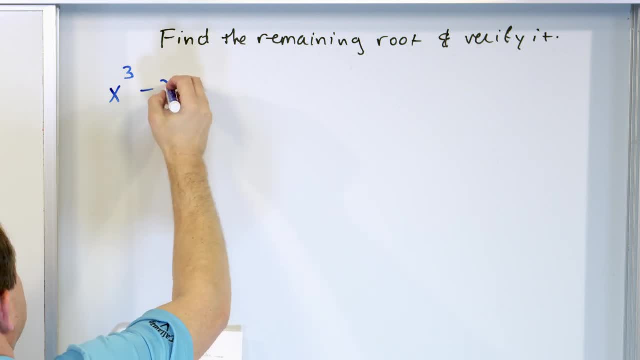 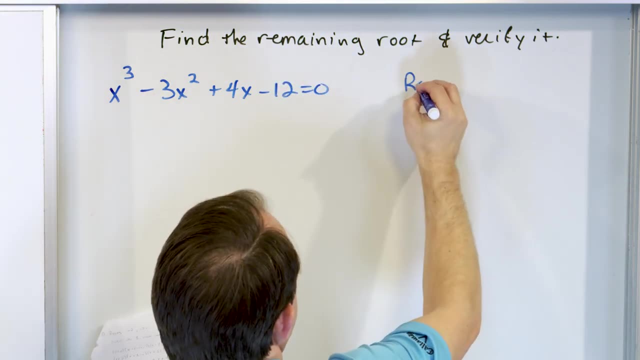 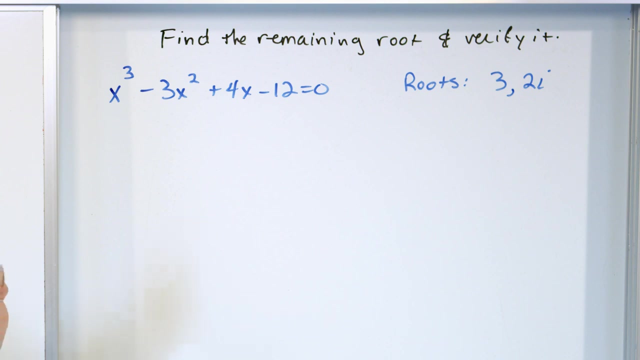 So the equation we have is x cubed minus three, x squared plus four, x minus 12,, zero, And the roots that I'm giving you here are three and two i. So the question says: find the remaining root and verify it. So what you're supposed to do here is look at the equation. 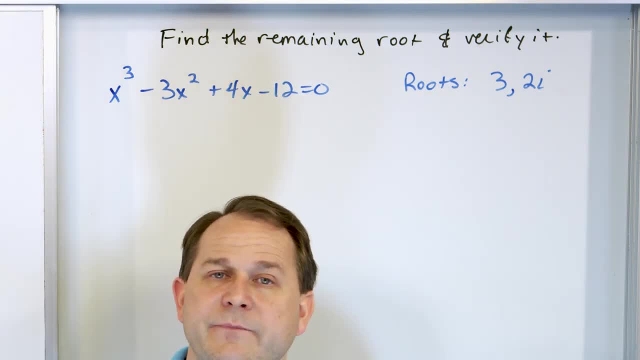 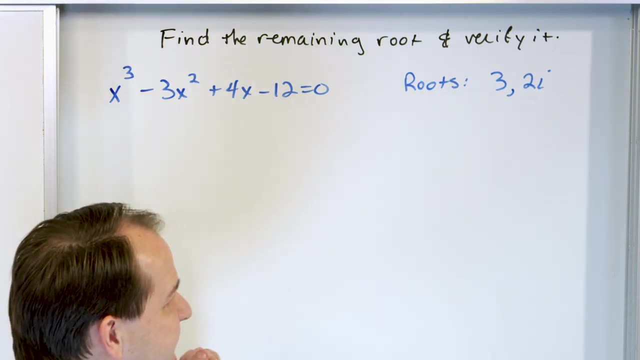 You see that it has a degree of three. That tells you it's a cubic equation. That tells you there's only three roots of this equation. Some could be real, Some could be complex. That's the first theorem we've learned. The second thing is I'm only giving you two of these roots, So you know. 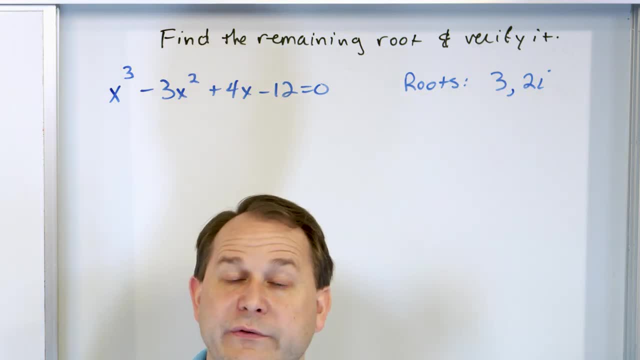 there must be a third one. You know that you have a two. i is one of the roots and you're going to have to verify it. You know that imaginary or complex roots always come in pairs, conjugate pairs. So if you know that this is a root, then you also then know that all of this. 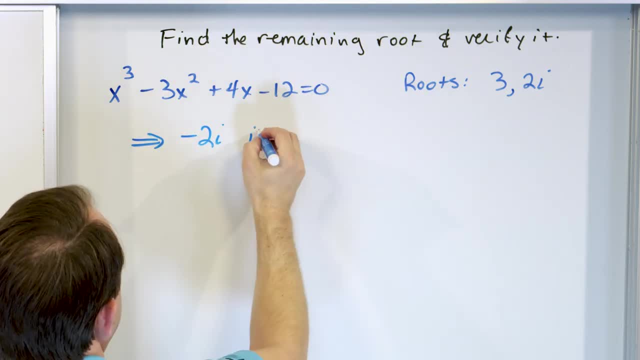 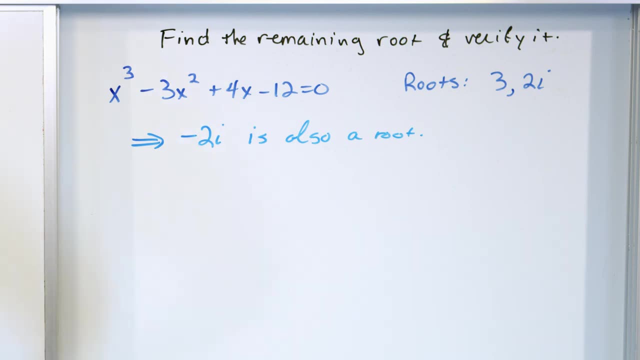 stuff kind of implies that negative two i, the conjugate of the two i, is also a root And they're asking you to verify that. There's a couple of ways to verify it. We've actually used synthetic division and things like this in the past, But the cleanest way to verify this is: 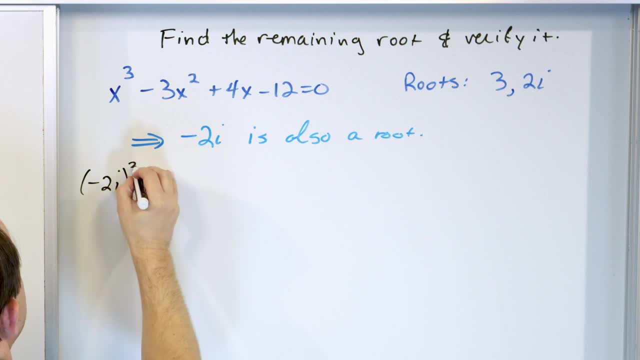 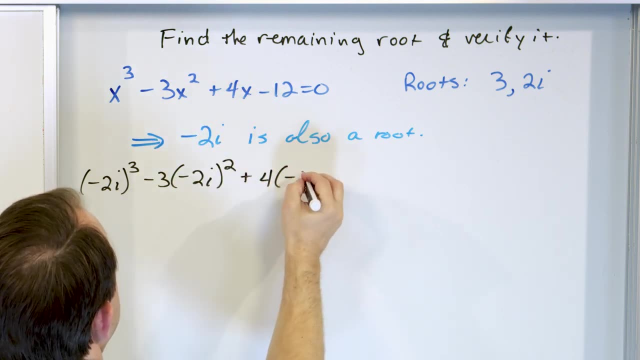 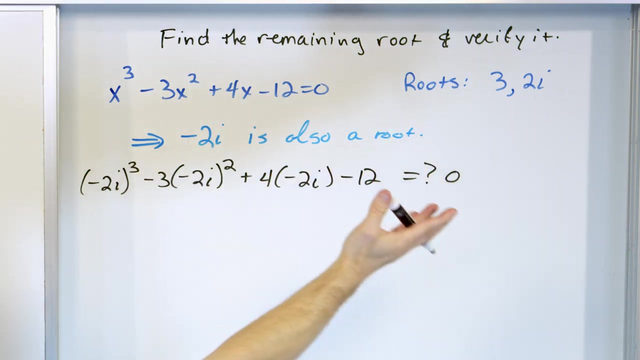 a root is to put it in here. So: negative two- i cubed, minus three x squared plus four x squared minus three. negative two: i squared from this term for negative two, i this term minus 12.. And we're asking ourselves, does this equal to zero? If it is equal to zero, then this is a root and 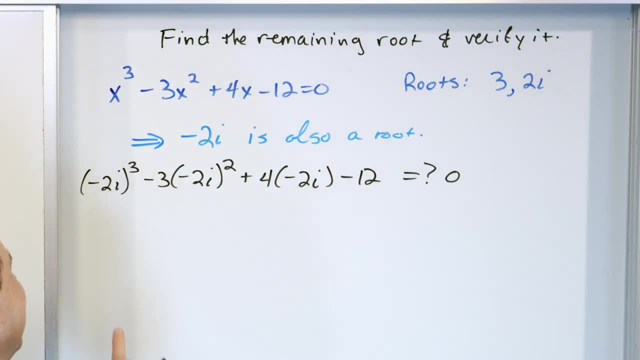 we've done everything correctly And so it's really easy to make mistakes here. because, notice, we have negative two i. The whole thing is cubed. So what happens is the cube applies to the sign, which is like a negative one out there, It applies to the two and it also applies to the 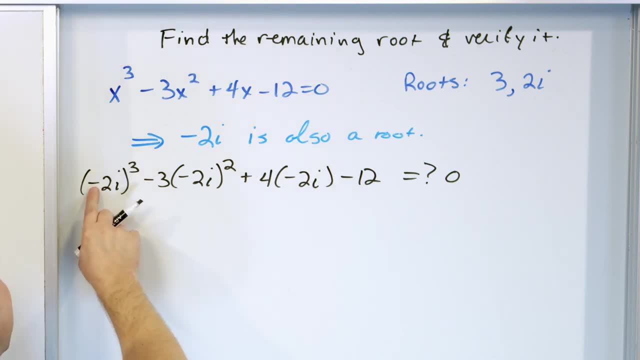 to the i right. So if you think about it, negative times, negative gives positive times. negative again would give you negative Two times two times two actually gives you eight, And then the i cubed. we're going to save that for later because if we try to do all the signs, 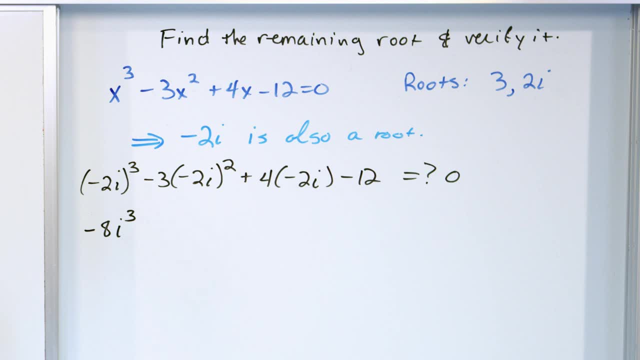 associated with the imaginary number at the same time as everything else. we're going to make a huge mistake eventually. So negative two times negative. two times negative two gives you negative eight- i cubed is this term- Then you have the negative three. Then on the inside, here again. 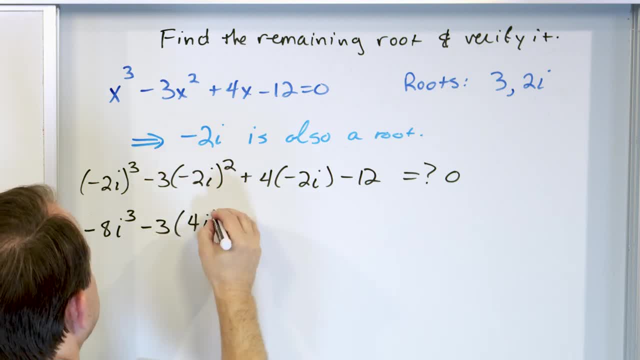 negative two times negative. two is positive. Negative three is negative. four i times i is i squared. We are not trying to. other students again will try to do all of this and also multiply by the negative three, all in the same step. 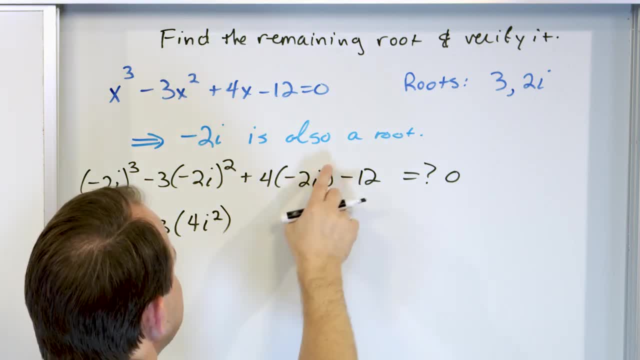 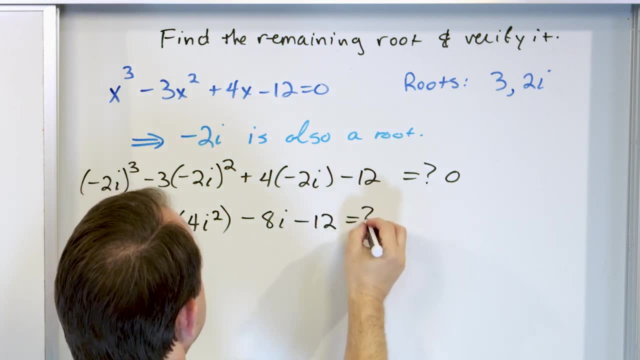 That's a huge mistake. You're going to make an error eventually. Now this one: there's actually no exponent, or the exponent is one. so I can multiply this Negative eight- i, And then I have minus 12.. Is that equal to zero? So over here I have negative eight. i cubed, I'm going to write. 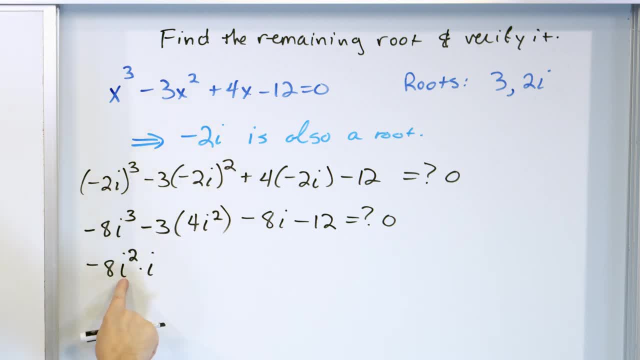 that as i squared times i. Why am I doing that? that i squared is negative 1, and in the next step I'll replace it with negative 1.. If you try to do i times, i times i, it often gets confusing what's going to happen? Just as an intermediate step. 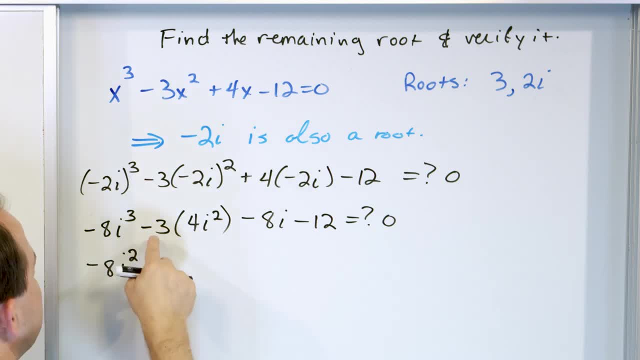 write it as: i squared times i. That's equal to i cubed right. This is going to be negative 12. i squared Again. I'm not going to do anything with the i's yet- And then I have negative 8i. 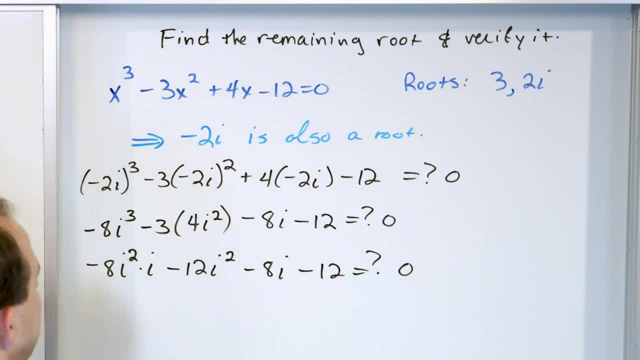 and I have minus 12.. Is that equal to 0?? Okay, what we have here is negative 8.. The i squared, now I can insert that that's equal to negative 1.. I still have an i there, and then I have minus 12.. 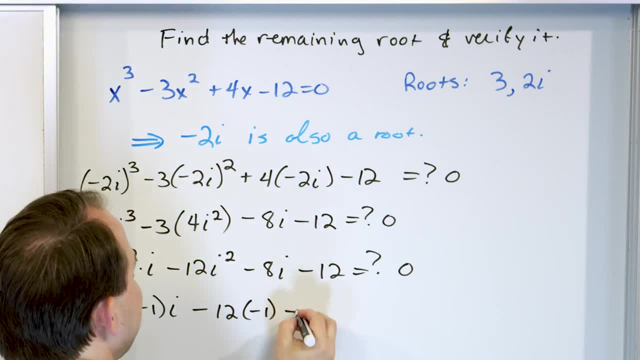 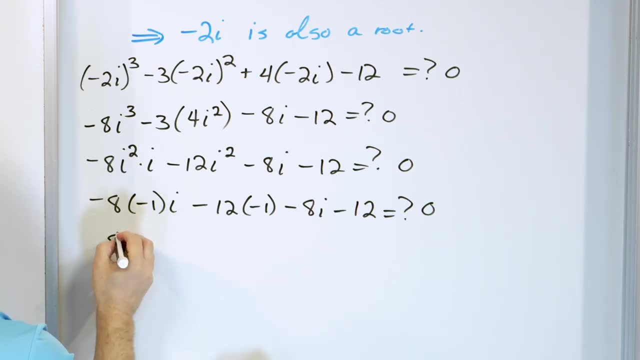 The i squared I can insert is actually equal to negative 1.. Then I have negative 8i, Then I have negative 12, and is that equal to 0?? So now I'm at the home stretch. This becomes positive 8i. 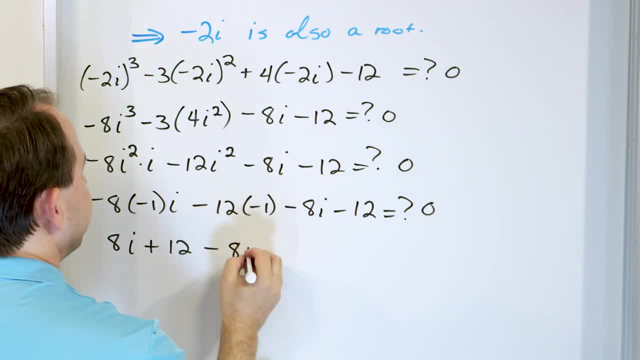 This becomes positive 12.. This is negative 8i and this is negative 12.. Is that equal to 0?? Well, you can see that the 8i and the negative 8i subtract to 0.. The 12 and the negative 12. 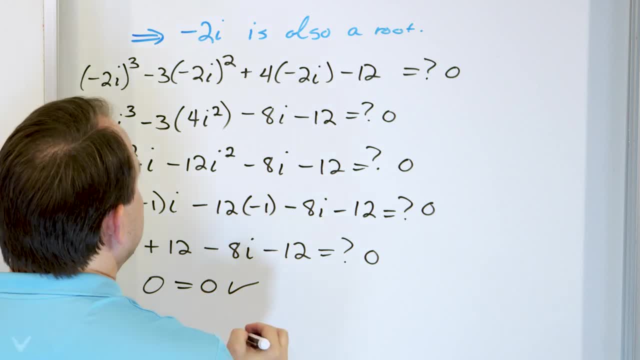 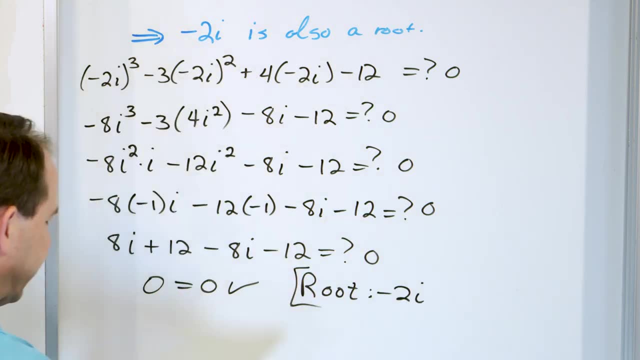 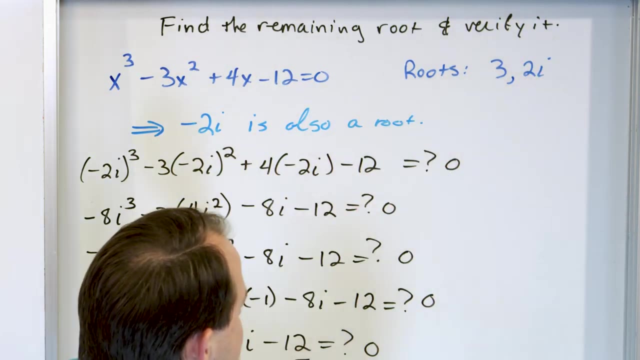 subtract to 0.. 0 equals 0 is a check. So what you have found, that a root or the remaining root is indeed negative 2i, which is what you're asked to do. The question said: find the remaining root and verify it, And we know from the conjugate root theorem that if this is a root, negative 2i must. 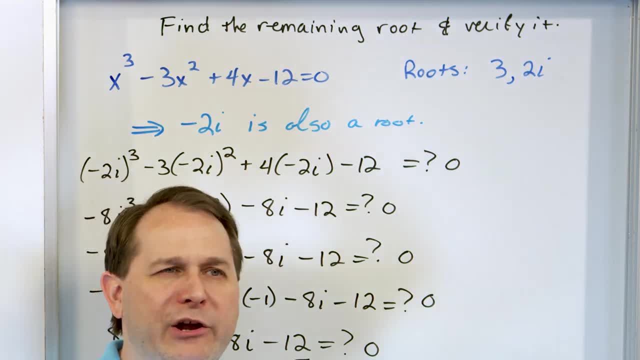 also be a root, And so we put it in here. And you might say: why do I crank through all of that and show you every little step to verify That the root is correct? Because, to be honest with you, there's a lot of places to make an. 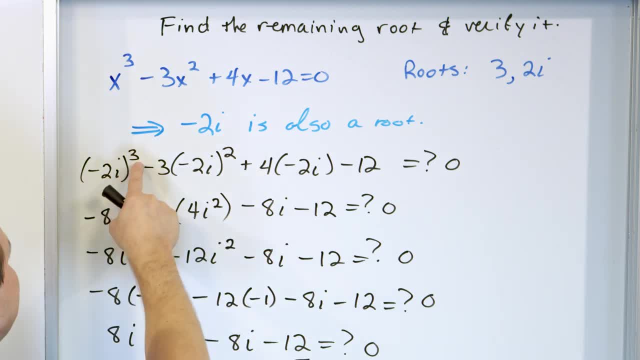 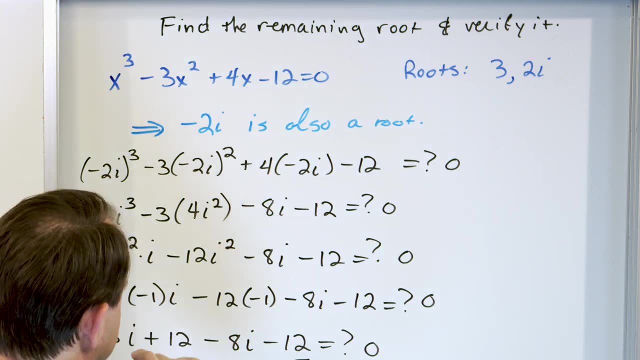 error here. when you have imaginary numbers, Most students will try to cube the negative 2 and then cube the i at the same time keeping track of all the signs in their head, and eventually make a sign error there. You can also do the same thing here, trying to. for instance, I had it right here. 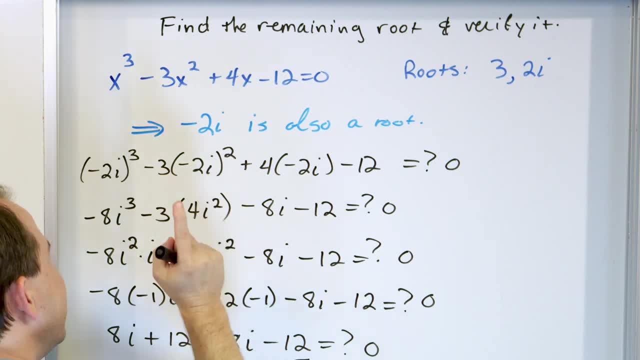 and I wrote it as negative 12i squared. But a lot of students will try to in their mind say, well, negative 12, and then this becomes a negative 1. That becomes a positive And they'll try to write it, do it all in their head.